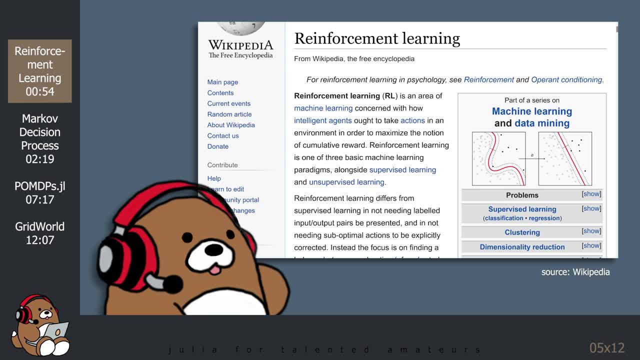 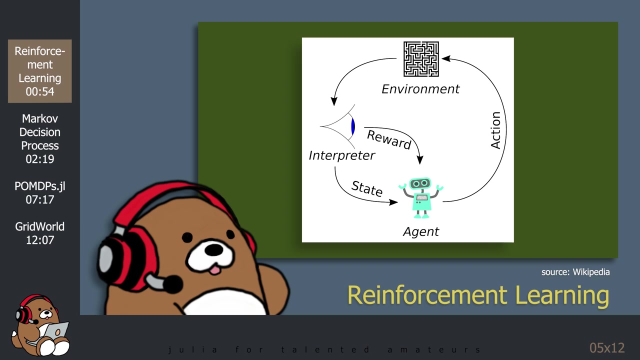 According to the Wikipedia article on reinforcement learning, reinforcement learning is the area of machine learning concerned with how intelligent agents ought to take actions in an environment in order to maximize the notion of cumulative reward Between supervised, unsupervised and reinforcement learning. reinforcement learning feels the most like artificial intelligence. 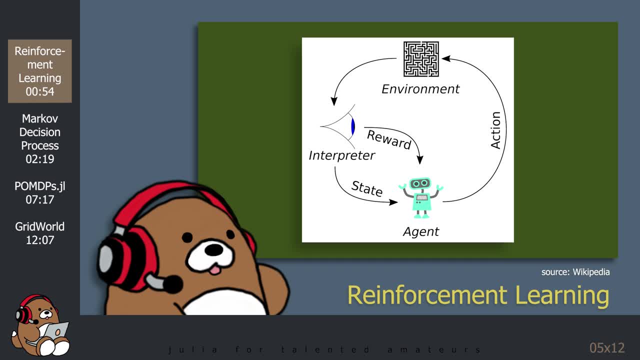 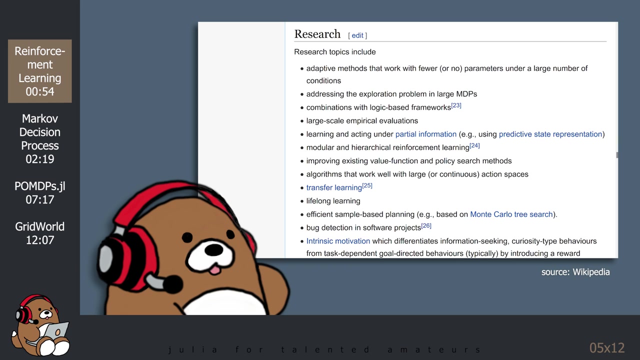 While supervised learning and unsupervised learning feel like a natural extension of data analysis and data science, reinforcement learning feels more like a natural extension of engineering science and social science. What Is Reinforcement Learning? Reinforcement learning is an enormous field of study with a rapidly developing body of literature, so I will only be providing 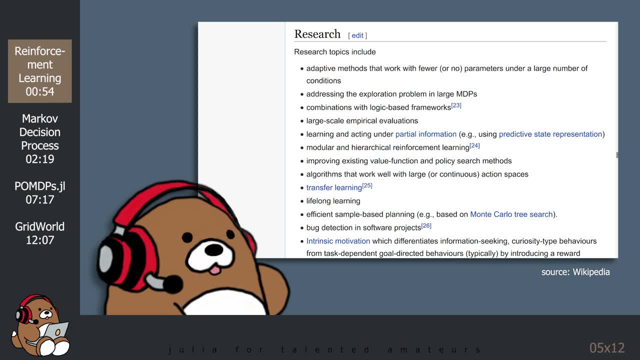 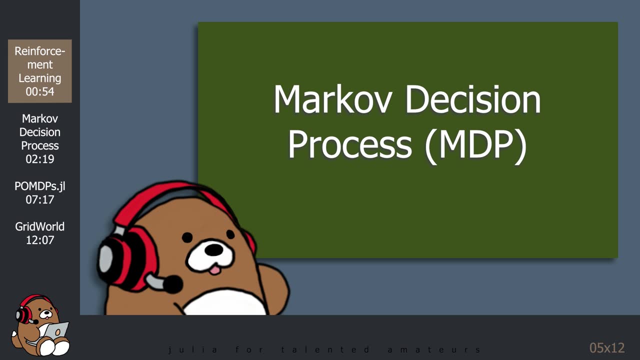 a brief glimpse into this world in this tutorial and the next tutorial. I hope to make a separate 13-part series dedicated to reinforcement learning at some point in the future. But before we can begin to think about reinforcement learning, we need to understand. 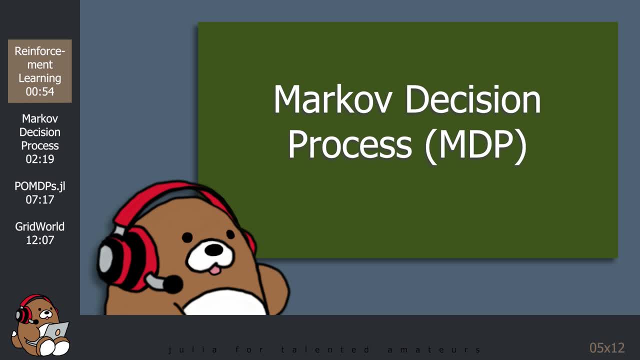 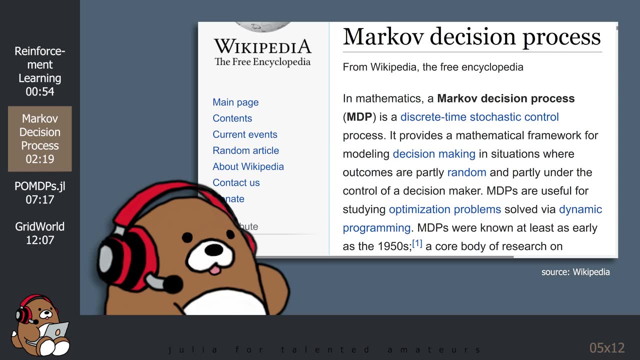 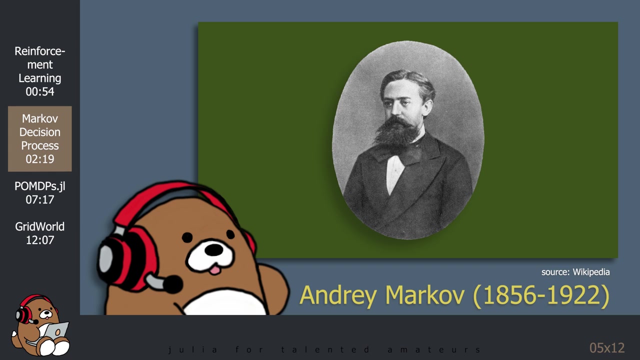 something called the Markov Decision Process. According to the Wikipedia article on Markov Decision Process, a Markov Decision Process provides a mathematical framework for modeling decision-making in situations where outcomes are partly random and partly under the control of a decision-maker. MDP is an extension of the Markov Chain, also known as the Markov Process. 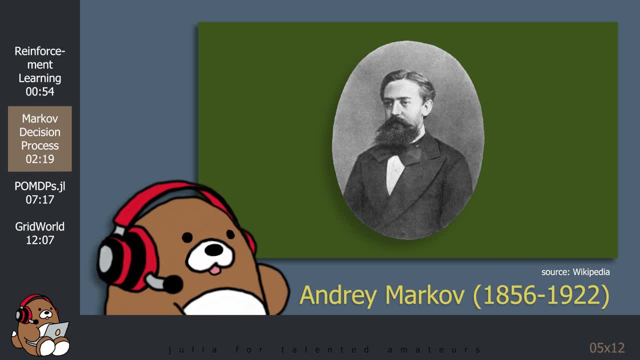 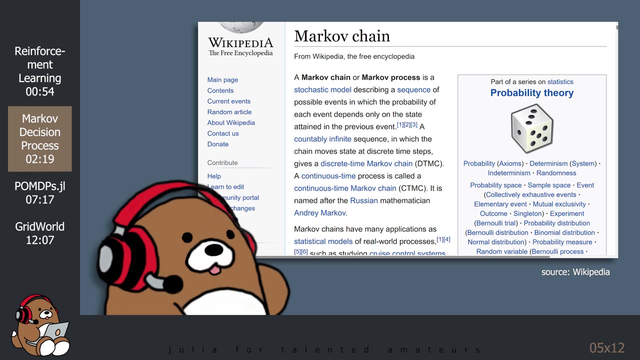 which was developed by the Russian mathematician Andrei Markov in the early 1900s. According to the Wikipedia article on the Markov Chain, a Markov Process is a process for which predictions can be made regarding future outcomes based solely on its present state. 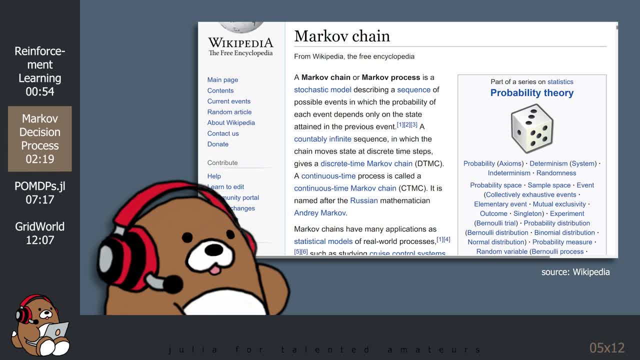 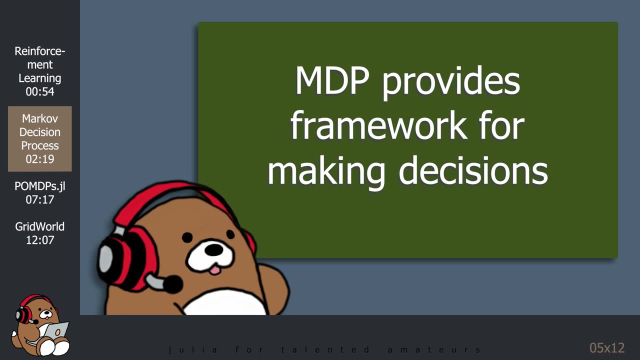 and, most importantly, such predictions are just as good as the ones that could be made knowing the process's full history. MDP takes the Markov Chain and formalizes it into a mathematical framework that may be used to make sequential decisions under uncertainty, where all of the uncertainty arises from outcomes. 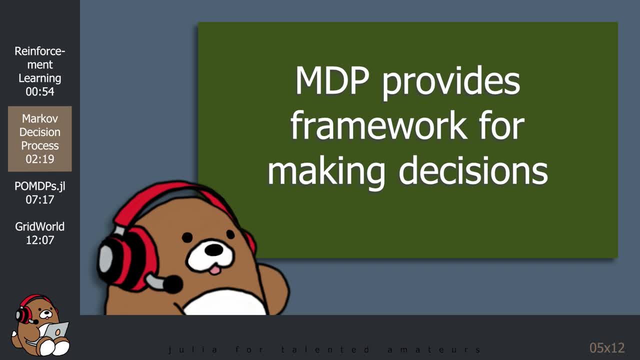 that are partially random and partially under the control of the decision-maker. MDP has been around since the 1950s and is used in many disciplines, including robotics, automatic control, economics and manufacturing. By itself, MDP is not considered reinforcement learning. 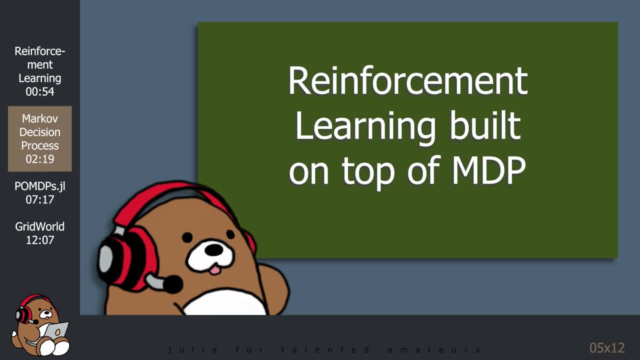 But MDP is the foundation upon which reinforcement learning is built, so knowledge of MDP is a prerequisite. Mathematically, MDP is a tuple containing five elements. S is a set of states called the state space. A is a set of actions, called the action space. 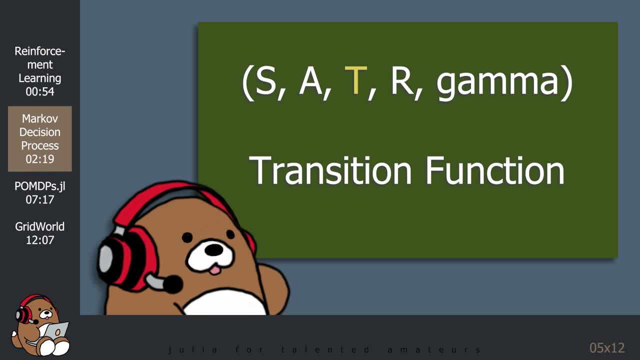 T is a transition function defining the probability of transitioning to each state given the state and action at the previous time. R is a reward function mapping every possible transition to a real reward value. Gamma is a discount factor that defines the relative weighting of current and future rewards. 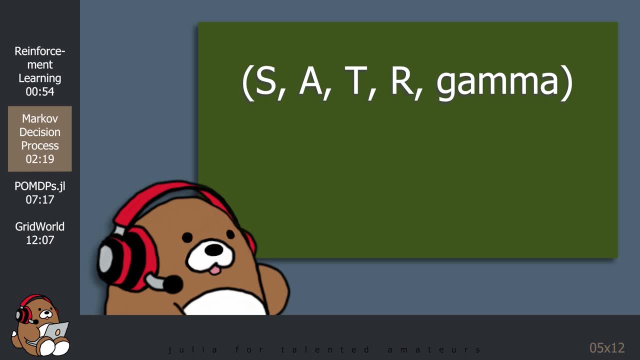 Don't worry about memorizing all of these elements. We'll see them again when we get to the code. This MDP is just a mathematical framework that defines a world where you can insert an intelligent agent. Once you've setup your MDP framework, the goal is to choose sequential actions that the intelligent agent can take in order to maximize the reward. 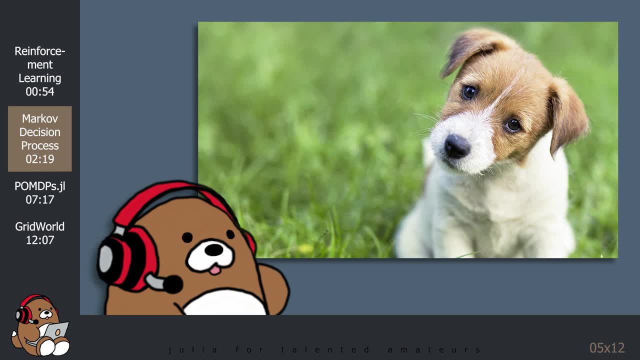 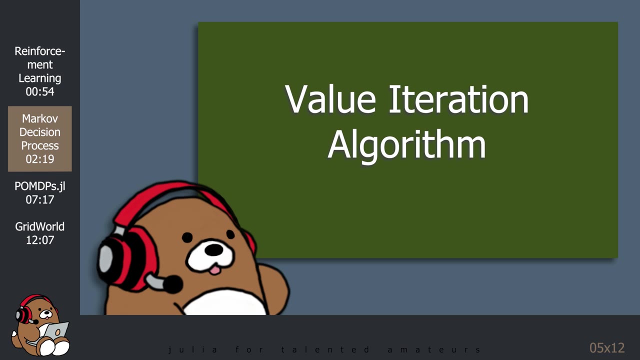 So how do we solve this MDP in order to find those sequential actions? For that reason, you don't need any of the other options available. You can use various algorithms to quote-unquote solve this MDP. The algorithm that we're going to use today is called Value Iteration. 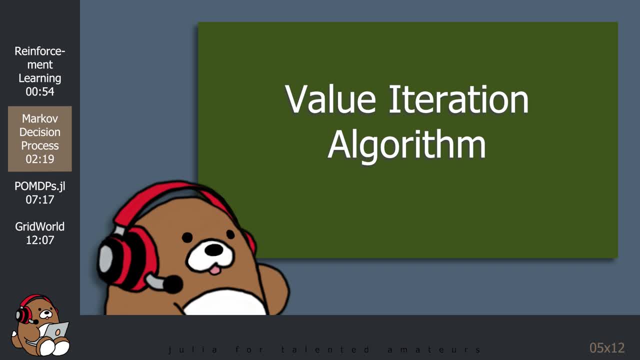 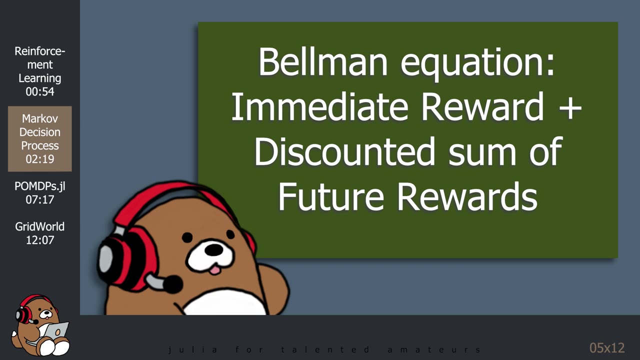 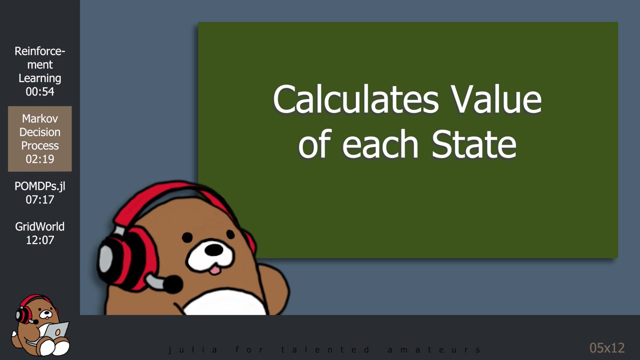 The Value Iteration algorithm uses an iterative process in order to calculate the value for each state, using something called the Bellman Equation. The Bellman Equation calculates the value of each state as the sum of an immediate reward plus the discounted sum of all future rewards. By using this equation, the Value Iteration- 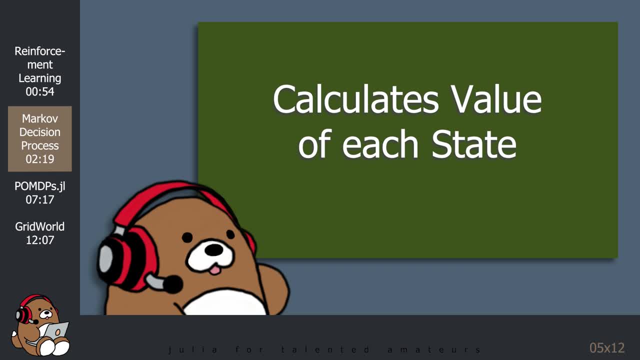 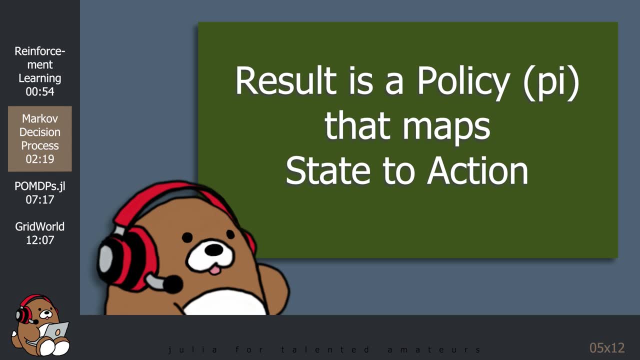 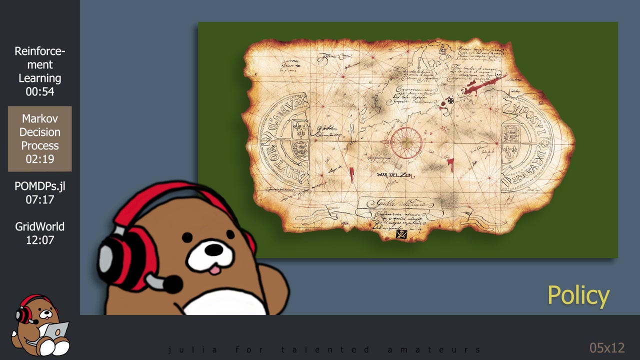 algorithm can figure out the optimal values for each state that maximizes the reward. Based on those values, the algorithm can then generate an optimal policy that maps each state to an action. The policy is referred to by the lowercase Greek letter pi. The policy is basically like a treasure map that tells the intelligent agent how to move around. 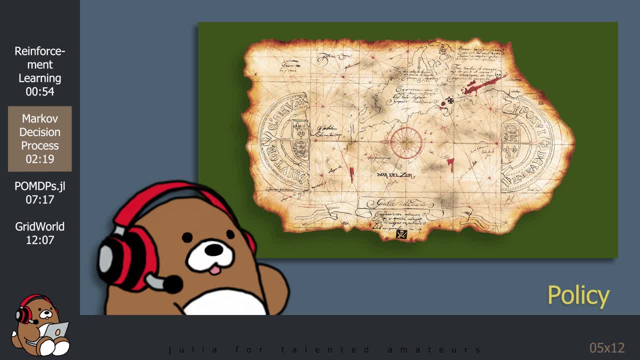 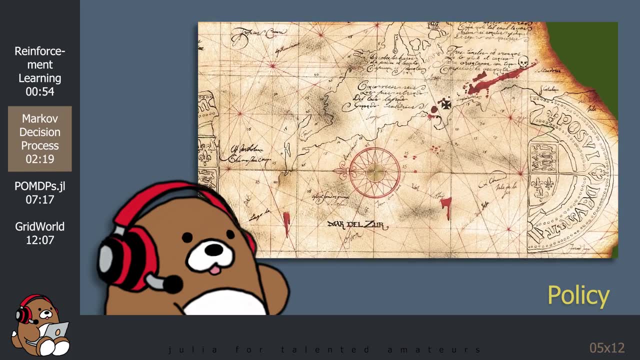 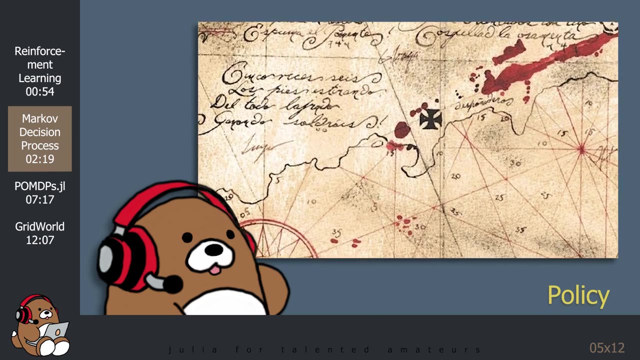 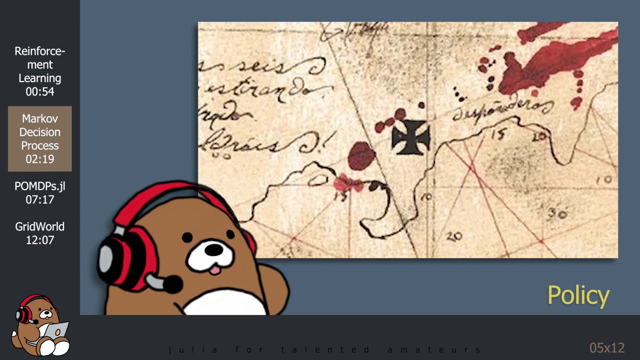 in this uncertain world in order to maximize its reward. Having access to such a map could be extremely valuable right? So how do we get our hands on such a map? In the Julia world, we can implement and solve MDPs using the pomdpsjl package. 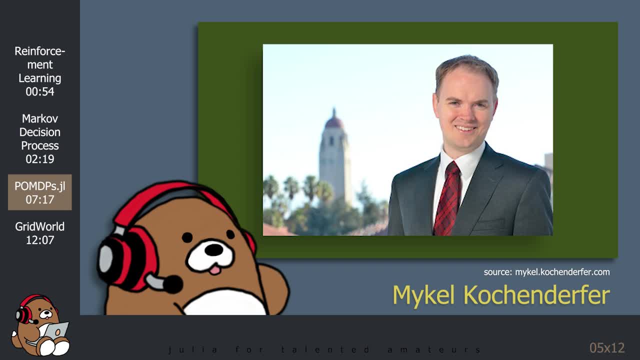 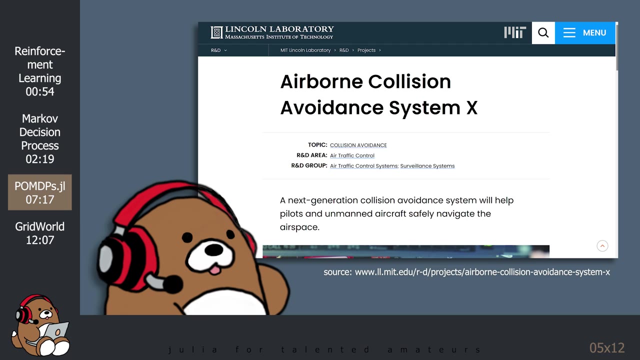 The pomdpsjl package can trace its roots back to the early days of Julia, when Michael Kochenderfer was working at MIT's Lincoln Laboratory in 2012.. He used an early version of Julia with the assistance of Julia co-founder Jeff Besantzen. 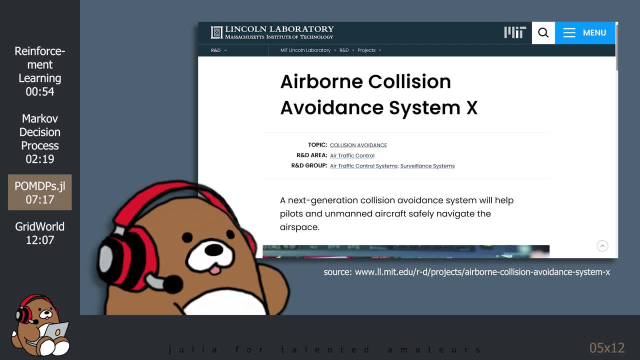 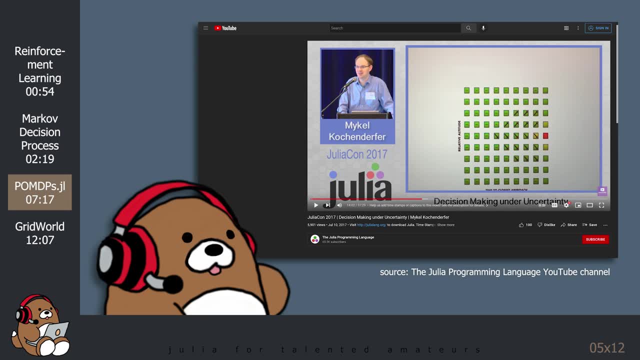 to develop code for a next-generation aircraft collision avoidance system to be used on all commercial airplanes. Michael Kochenderfer gave a fascinating presentation on the subject at JuliaCon 2017.. If you haven't seen it yet, I highly recommend watching it. 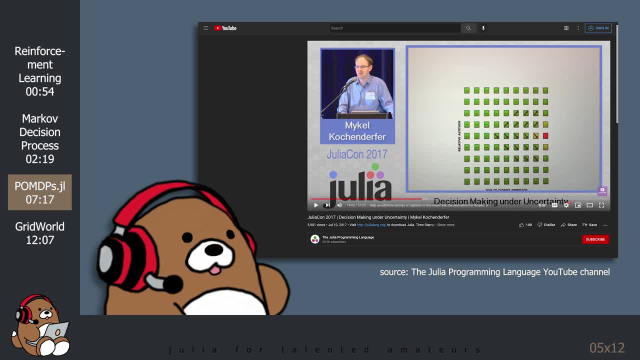 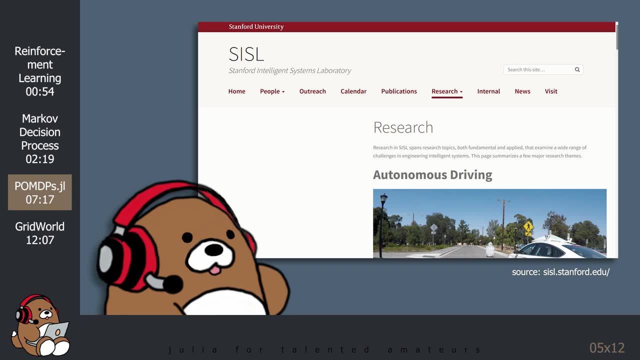 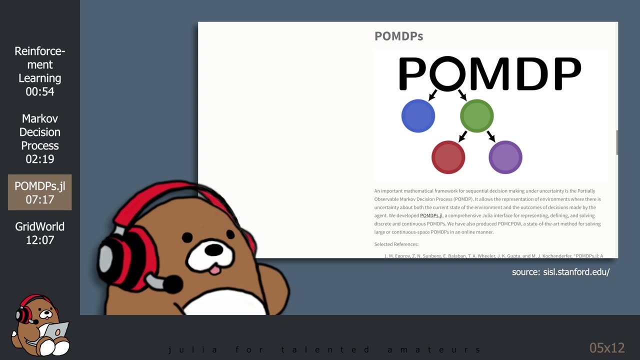 There's a link to it in the description. Michael Kochenderfer is currently an associate professor at Stanford University and the director of the Stanford Intelligent Systems Laboratory. The pomdpsjl package is a product of that lab, developed by a team led by Zachary Sundberg. 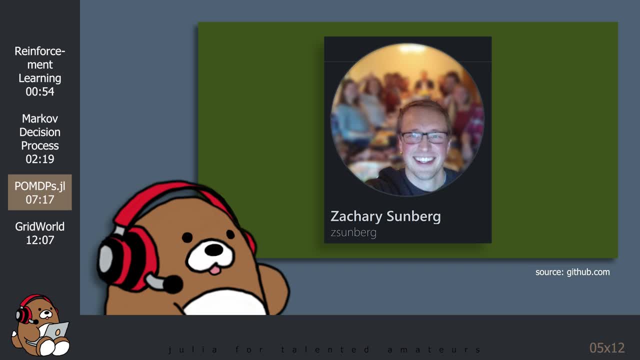 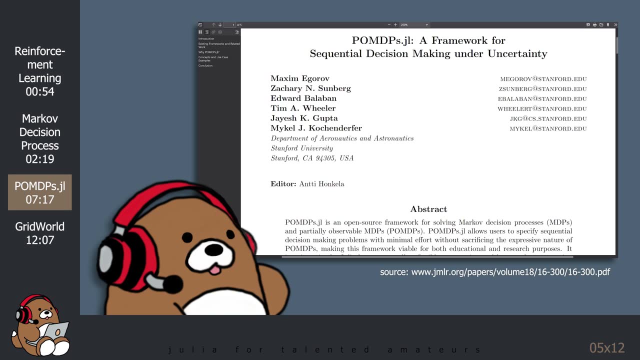 who was a Stanford PhD student at the time the package was created. The team published a paper in 2017 titled POMTPsjl: A Framework for Sequential Decision-Making Under Uncertainty, with credit given to Maxim Igorov, Zachary Sundberg, Edward Balaban, Tim Wheeler, Jayesh Gupta and Michael 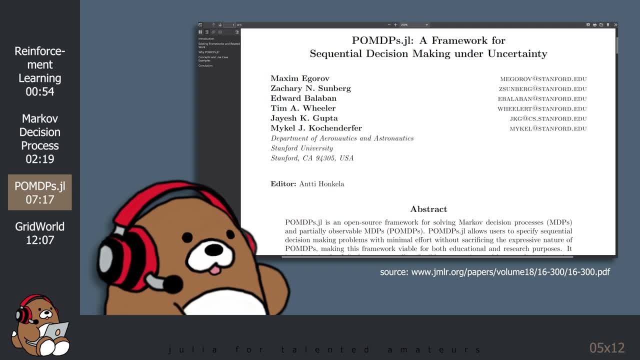 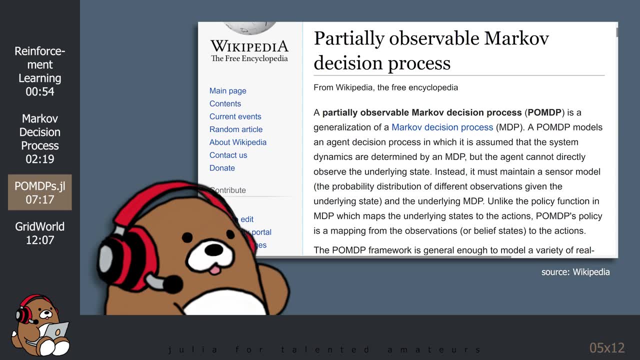 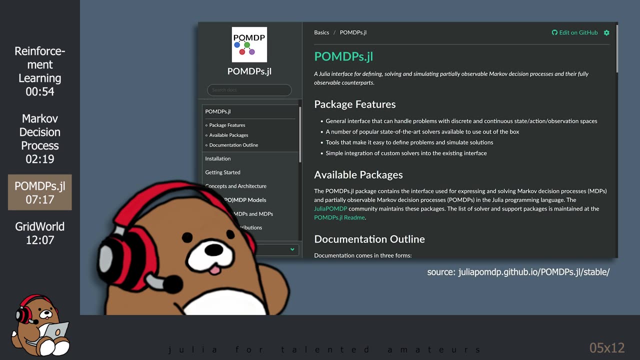 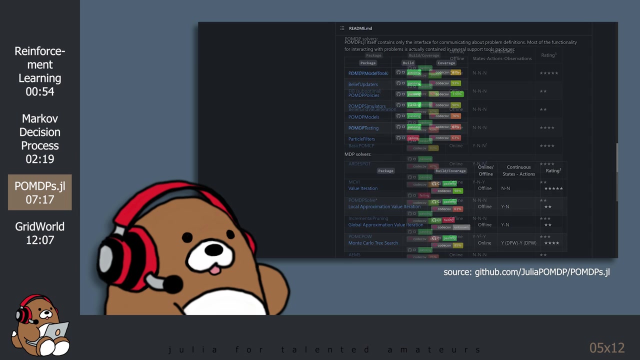 Kochendorfer, I apologize if I mispronounced any names. POMTP stands for Partially Observable Markov Decision Process. POMTPsjl is not a single Julia package, but instead it's an interface that works with an ever-expanding universe of complementary packages that are under active. 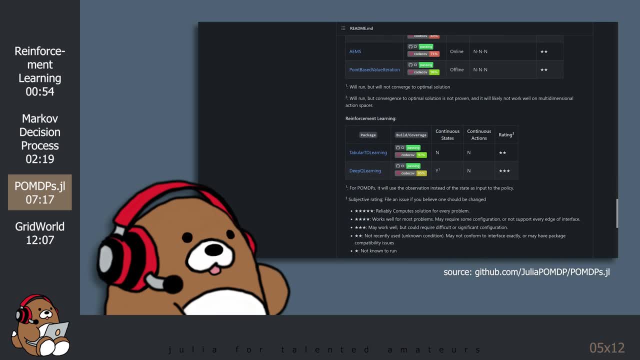 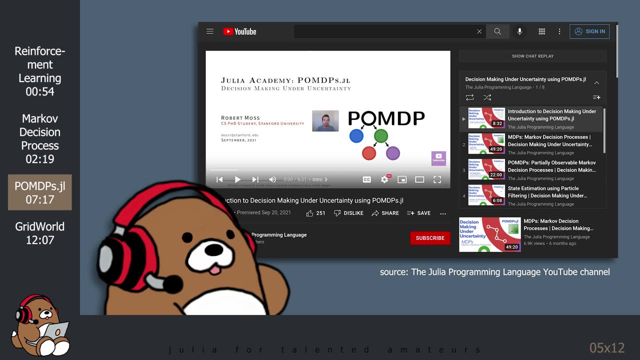 development by a lot of folks, many of whom are not familiar with POMTPsjl. There's a great tutorial playlist for the POMTPsjl package on Julia's official YouTube channel, hosted by Robert Moss, who is currently a PhD student at Stanford. There's a link. 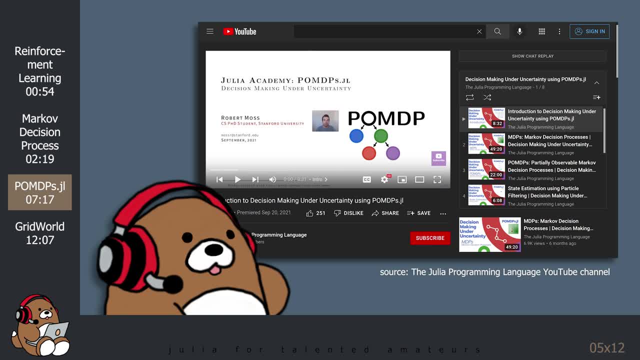 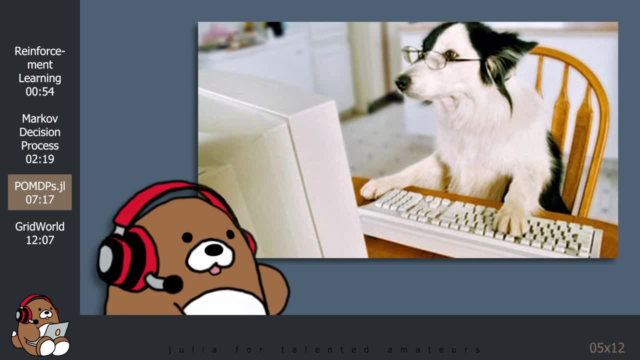 to that playlist in the description below. Just a fair warning though: POMTPsjl is not for the faint of heart. This is definitely not the case. It's not a beginner-level package, It's an intermediate-to-advanced-level package. that 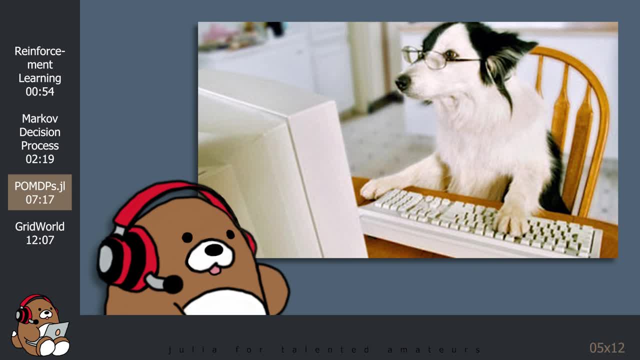 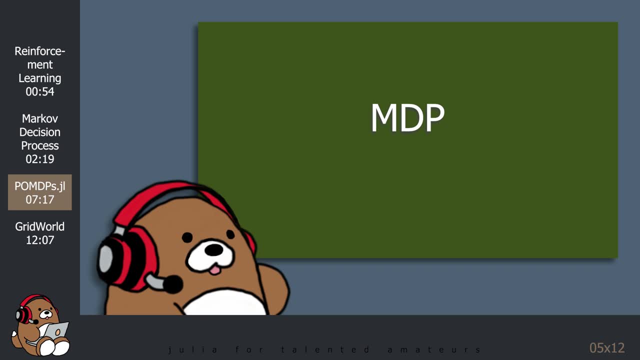 is still under active development. You can use the POMTPsjl ecosystem for many different applications, but we're going to use it today in order to implement and solve an MDP. For this section, knowledge of Julia and VS Code is required. 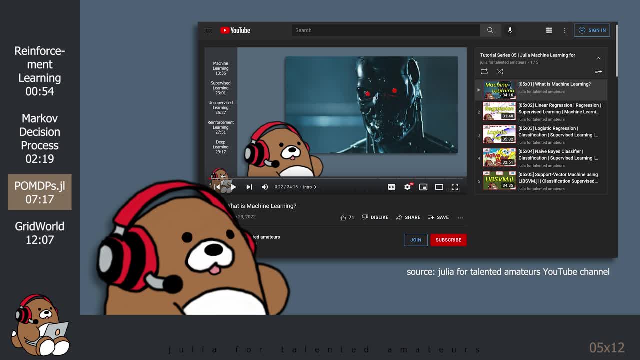 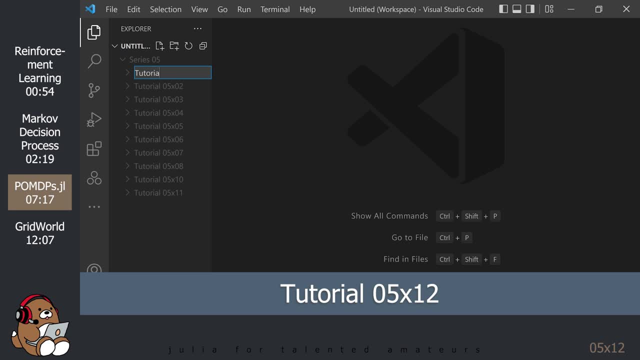 I'm also assuming that you're watching this entire machine learning playlist In your VS Code Explorer panel. create a new folder for this tutorial In the tutorial folder. create a new file called rl underscore, mdp dot jl. Launch the Julia REPL by using Alt-J, then Alt-O. 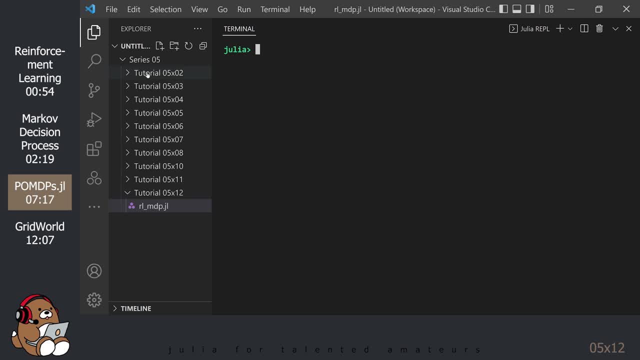 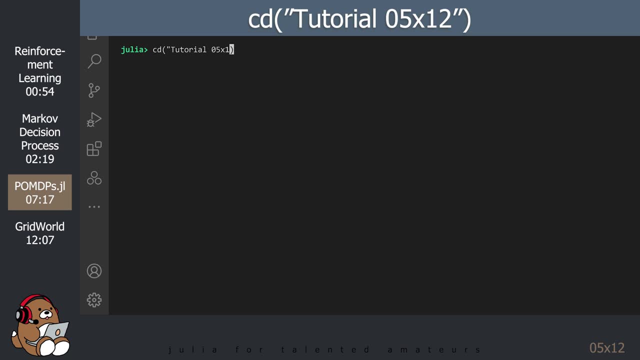 Maximizejl. Maximize the REPL panel In the REPL. change the present working directory to your tutorial directory. Enter the package REPL by hitting the closing square bracket. Activate your tutorial directory. Add the following packages: Discrete Value Iteration. 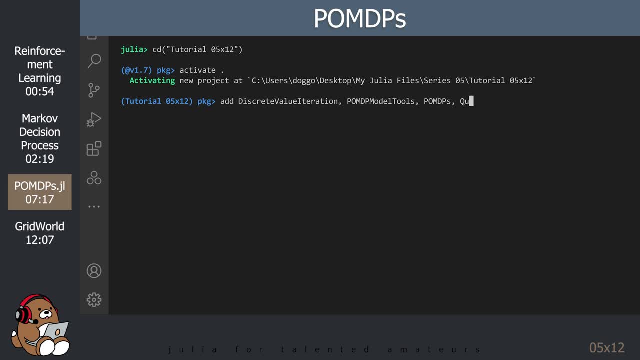 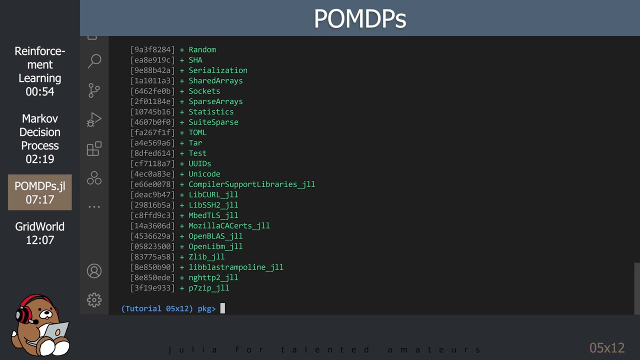 POMDP Model Tools, POMDP Methods and QuickPOMDPs. When adding these packages, pay close attention to the uppercase and lowercase spellings. POMDPs: uses uppercase P-O-M-D-P but uses a lowercase s. 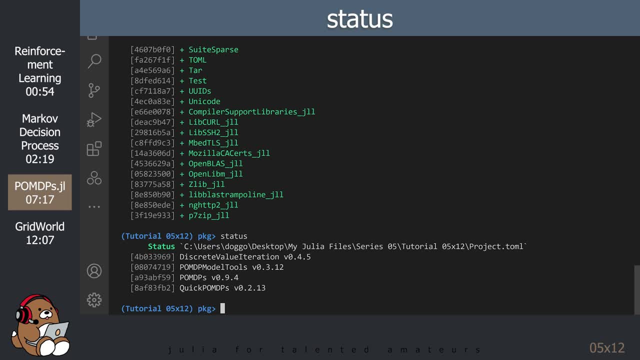 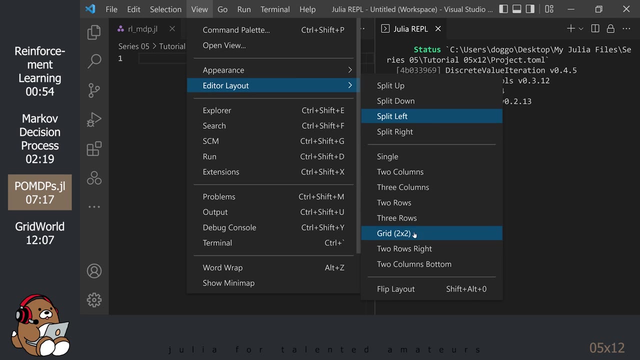 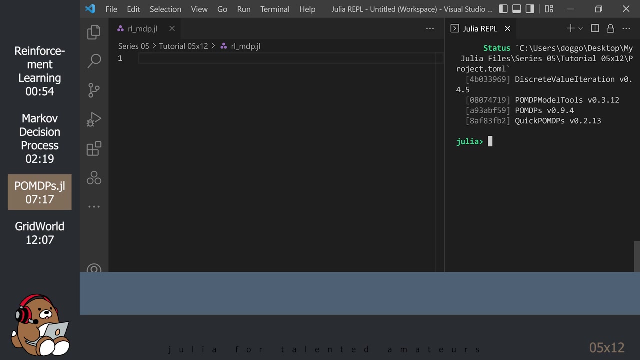 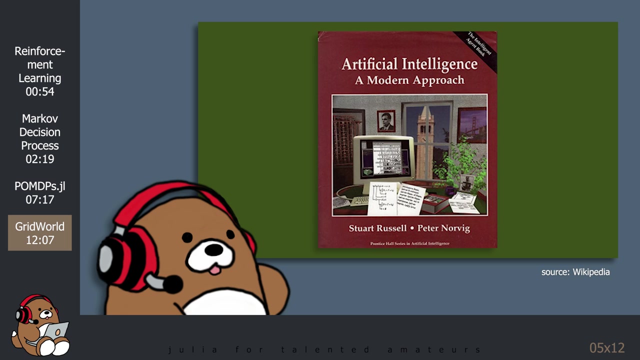 Type in status to confirm the version numbers. Access the Package REPL by hitting Backspace. For this tutorial, I'm going to dock the REPL panel next to my Editor. OK, let's take a look at a motivating example. Today's motivating example is inspired by an example found in the textbook. 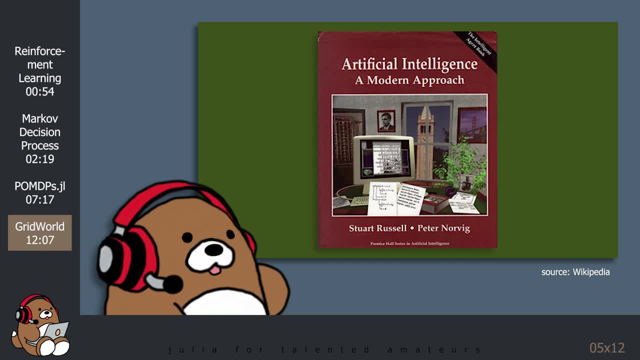 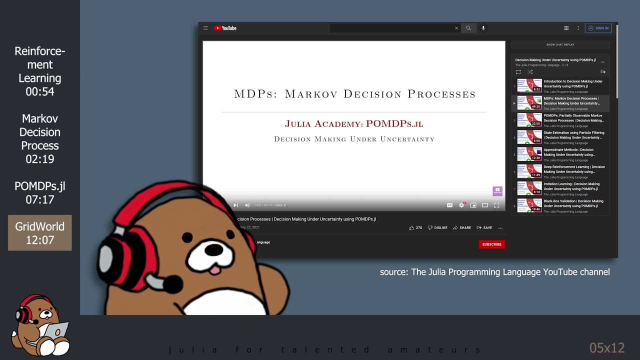 Written by Stuart Russell and Peter Norvig called Artificial Intelligence: A Modern Approach. I've modified the example slightly for this tutorial. The actual code for this example comes from Robert Moss' tutorial on MDPs. I've modified his code slightly in order to simplify it a little bit for this tutorial. 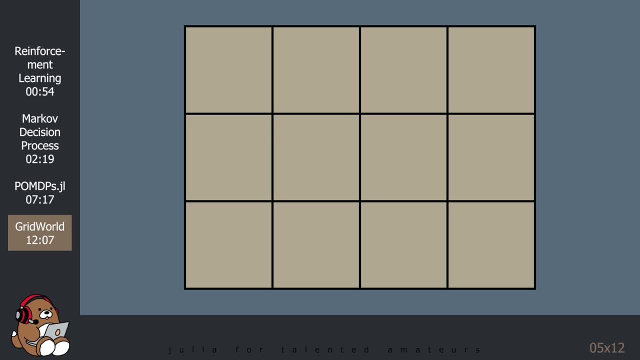 So here's the basic setup and objective. Our world, or environment, consists of a 12-tile grid with 3 rows and 4 columns. Each tile is identified by an x-y pair, with tile in the lower left corner and tile in the upper right corner. 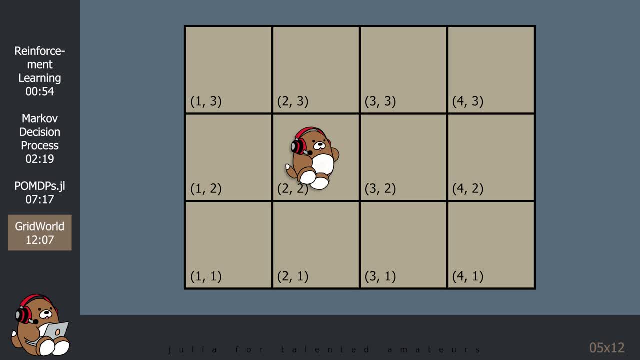 In this environment we're going to place an intelligent agent- Let's call him Agent Doggo- That can move from tile to tile, But when the agent moves there's some uncertainty. For example, if the agent needs to move up, there's only a 70% chance that the agent 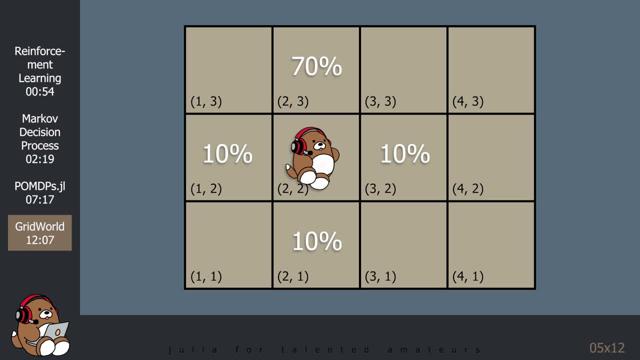 will actually move up. There's a 10% chance that the agent may move left and a 10% chance the agent may move right, and there's another 10% chance that the agent may move down. Also, in this example, we're going to use a 10% chance that the agent will actually move. 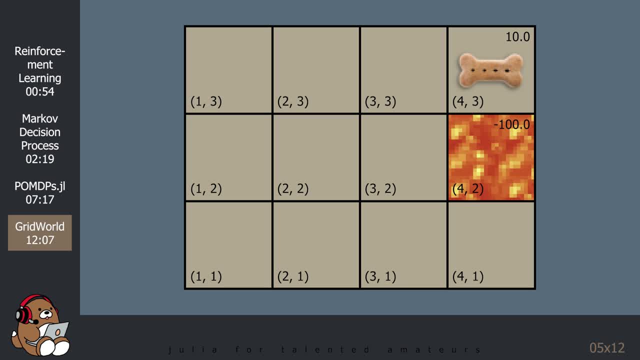 up In this environment. there are a couple of rewards, One positive and one negative. The positive reward is a doggo biscuit worth 10 points located at tile. The negative reward is a lava pit worth negative 100 points located at tile. 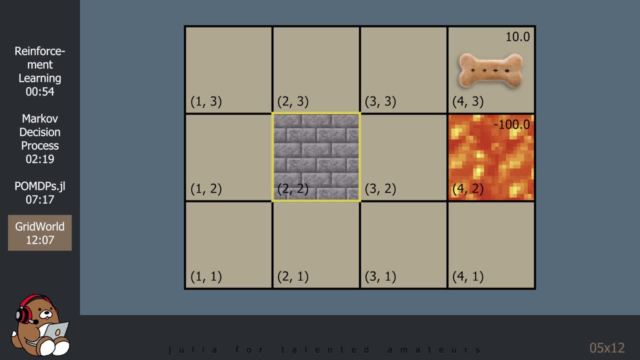 And just to keep things interesting, there's an obstacle located at tile. This obstacle is called the lava pit, So let's go over it one more time with this example that we just saw in the demo. Okay, so the doggo biscuit is located at tile. 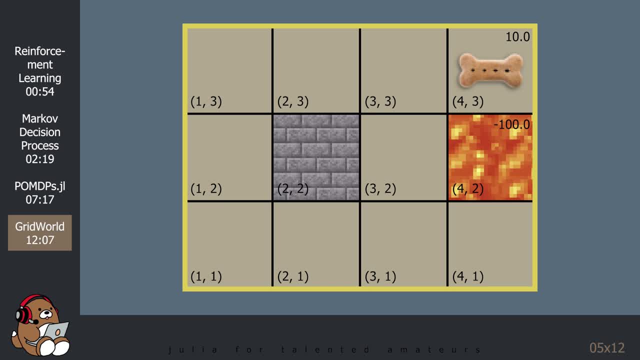 It just needs to move. And if the agent moves up to tile, it can move up at tile. And if the agent does not move up to tile, it can move up at tile. Also, if the agent does not move up to tile, it can move up at tile. 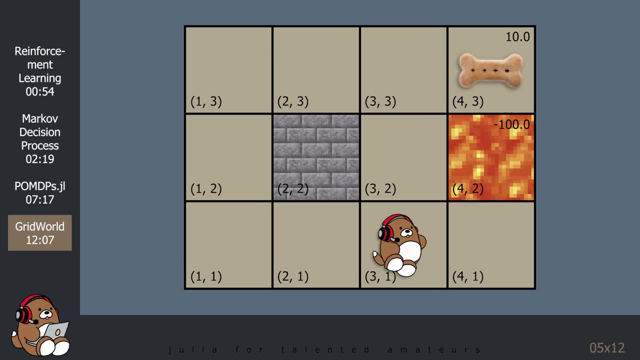 So we have here that the agent does not move up to tile 2, that the agent cannot pass through. Also, the agent cannot move beyond the borders. So if Agent Doggo starts at tile, which path should he take in order to get? 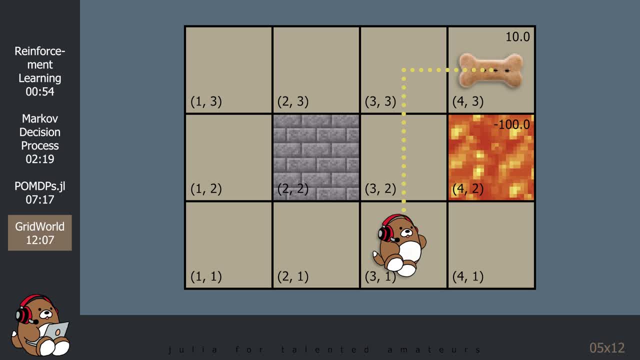 through the doggo biscuit. Intuitively you might think that the agent should take the shortest path, But then there's a slight risk that the agent will fall into the lava pit. D pleasure will fall into the lava pit. The alternative is to take the long way around, which is safer but will take more time. 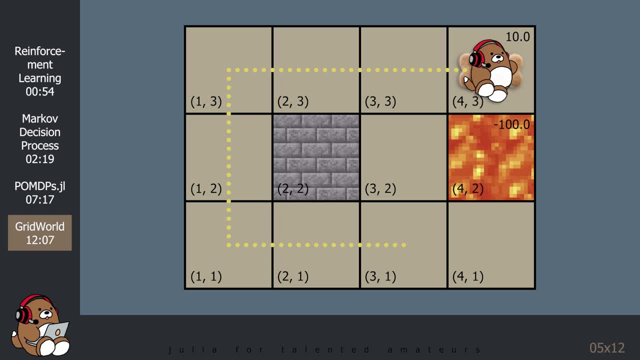 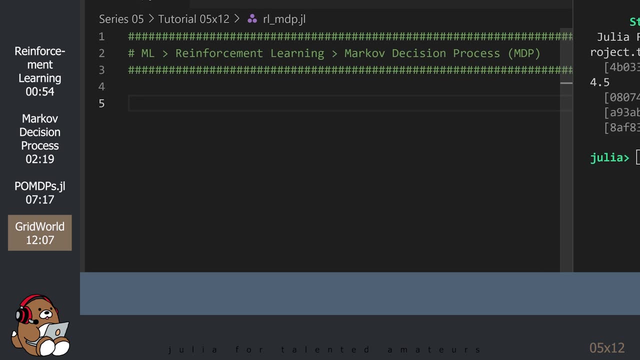 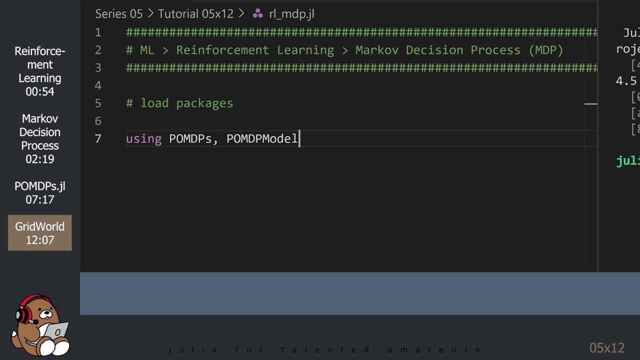 So what should Agent Doggo do? This is a classic example of decision-making under uncertainty. Let's see how we can use the pomdpsjl package to solve this problem. First, we need to load our packages. Since the pomdpsjl package is really just an interface, we need to load several additional. 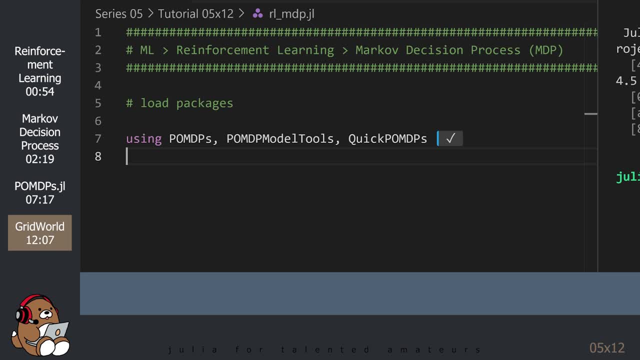 packages in order to use it. The additional packages that you need to include will depend on the problem that you're trying to solve. The actual solver is stored in a separate package. That's because there are many different solvers that you can use with the pomdpsjl. 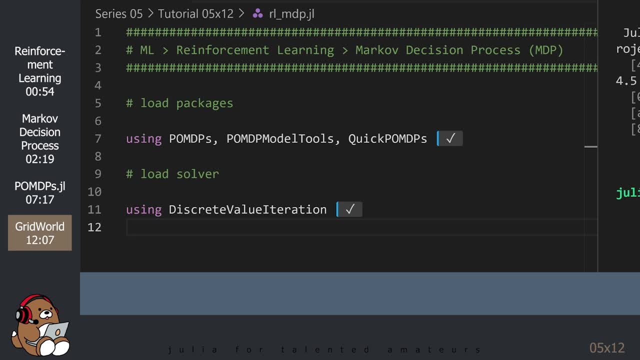 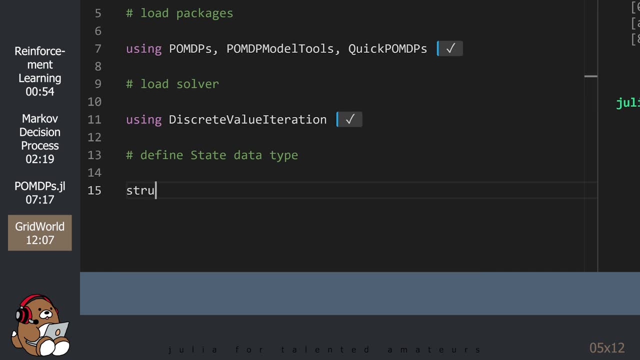 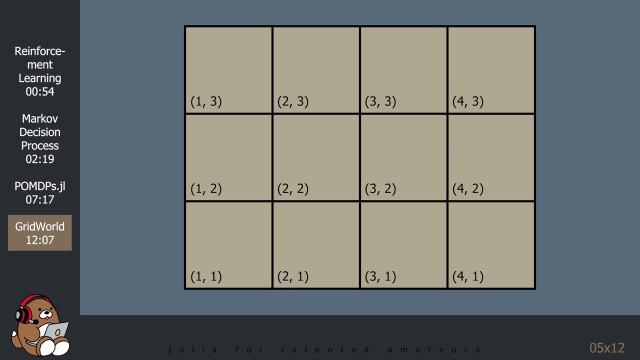 interface. The solver you choose will depend on the problem that you're trying to solve. Next, we need to define a custom data type for the state. In our diagram, each state is the same as each tile, which is identified using an xy. 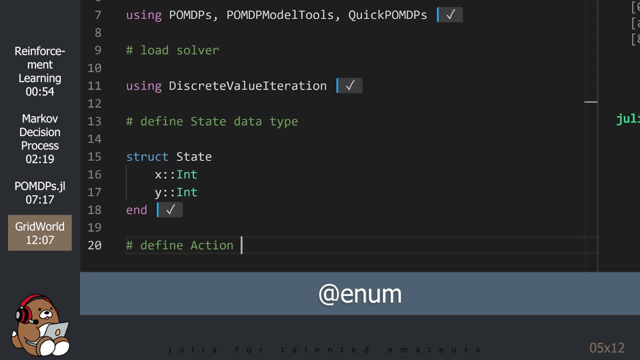 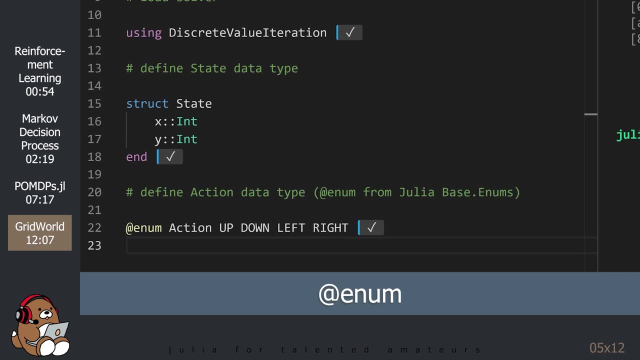 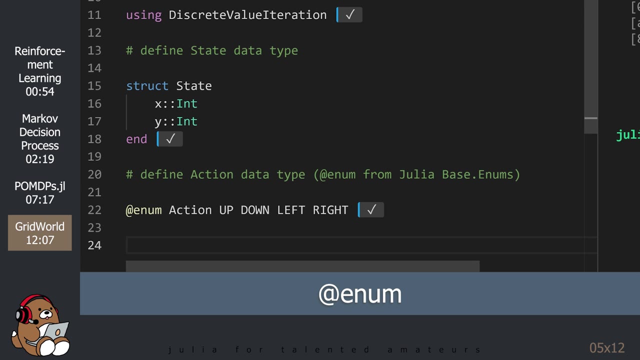 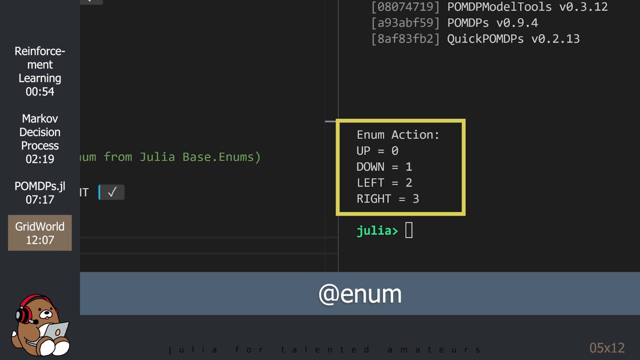 pair. Next, we need to define a data type for each action. For example, let's define an action that our agent can take. The at enum macro is from Julia Bayes. It creates a new data type for action. If you look in the REPL, you'll see that action contains the four directions, along with an. 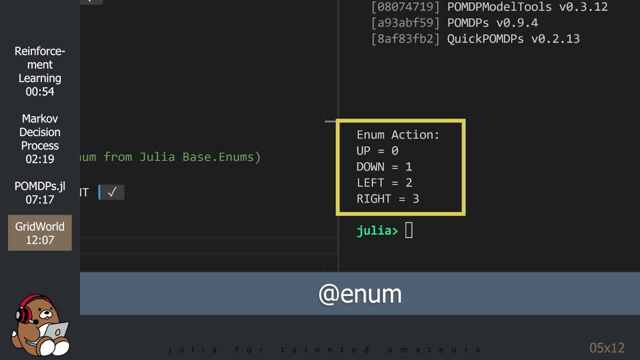 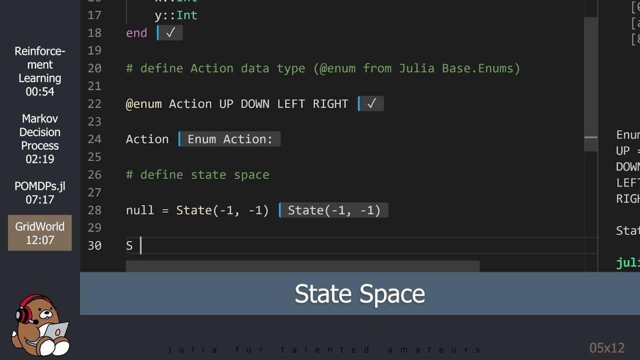 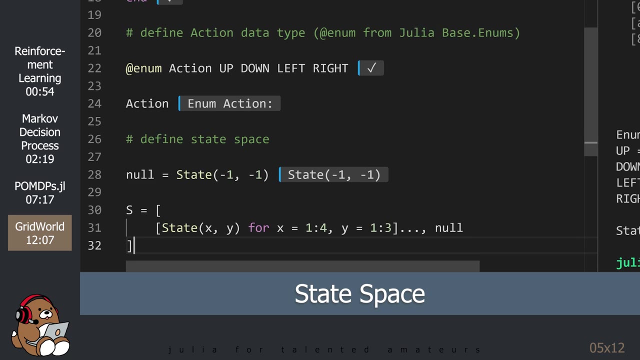 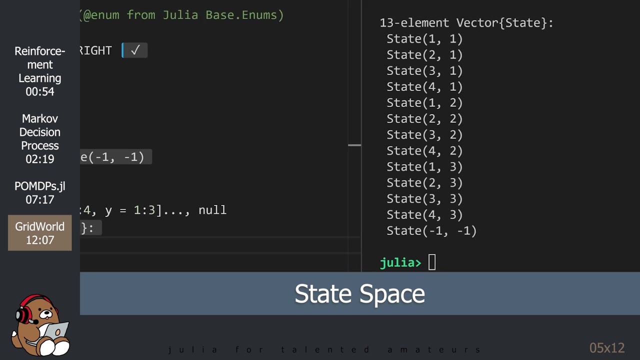 index number. For some reason, Julia starts the index at zero. Okay, Next we need to define the state space. The state space is just a collection of the 12 tiles plus one additional tile for something called a null state. The null state is used to end the game. 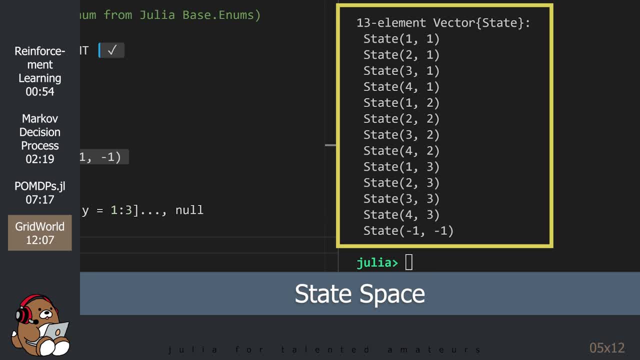 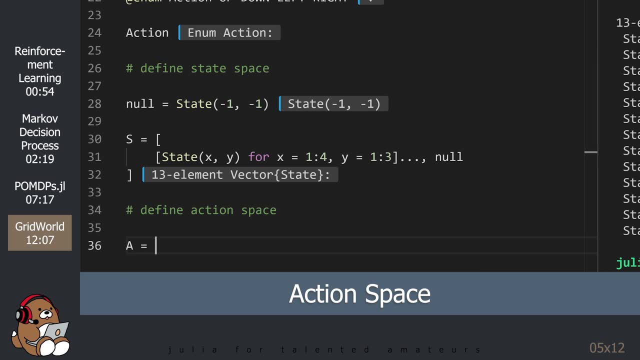 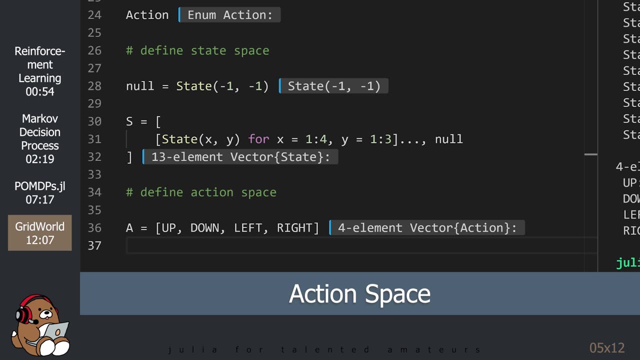 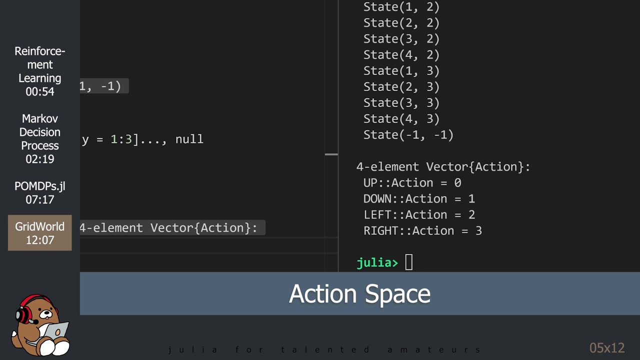 If you look in the REPL, you'll see that this code created a vector of all of the individual states. Next, we need to define the action space. You may be wondering: didn't we just do this? Well, no, When we used the at enum macro, we were setting up a new data type called action. 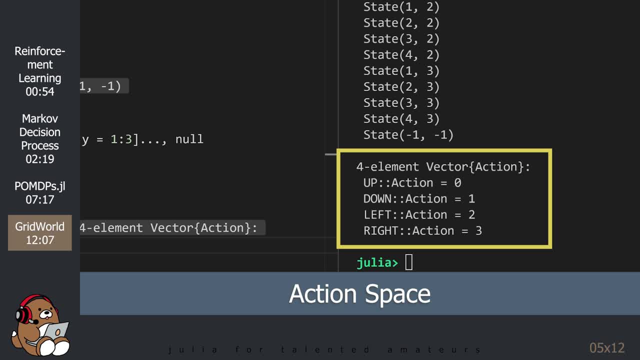 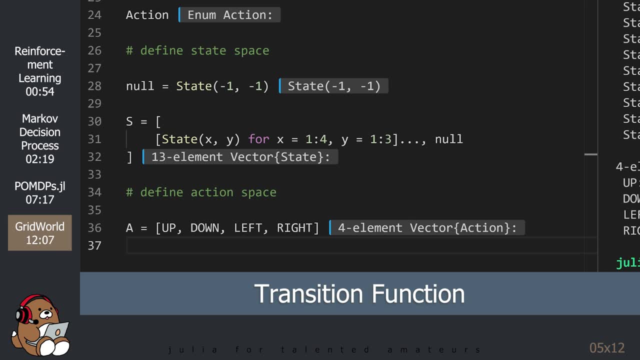 Here we're placing the individual actions into a vector of type action. Next, we need to define the transition function. This is the function that governs how the agent transitions from one state to another state, given some action. I'm not going to lie. this bit of code is the most difficult part of this tutorial. 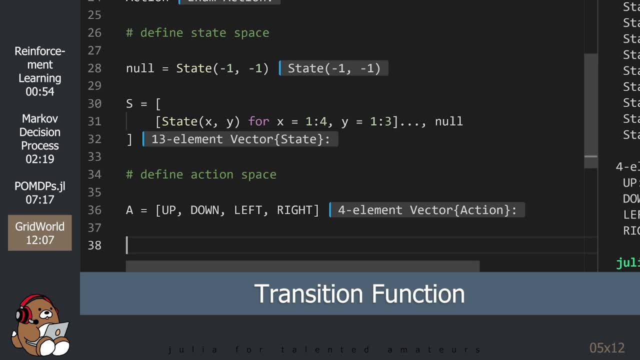 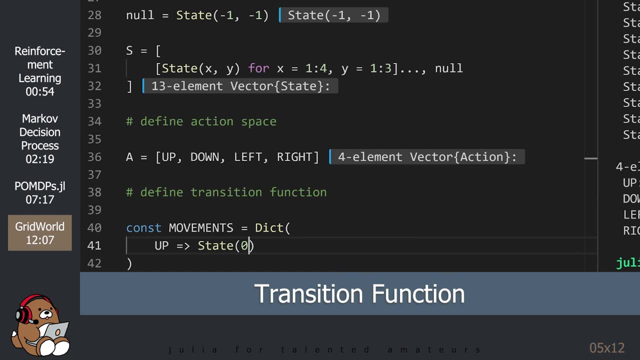 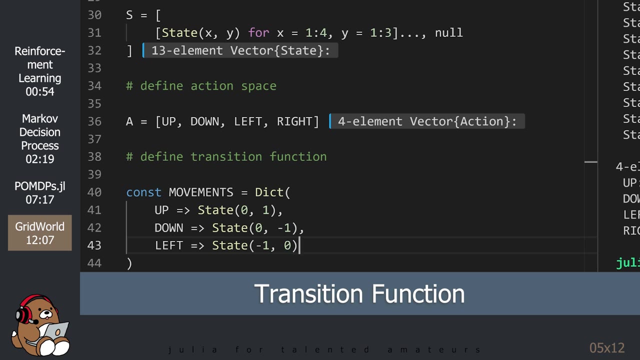 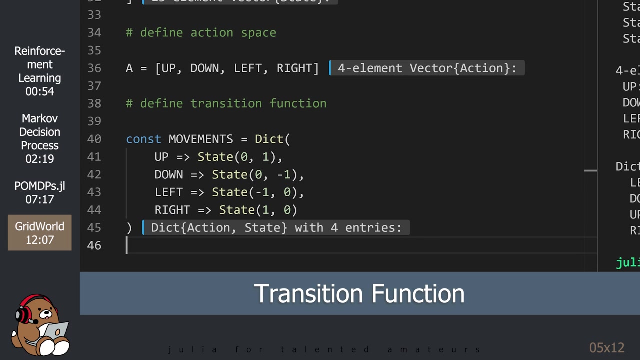 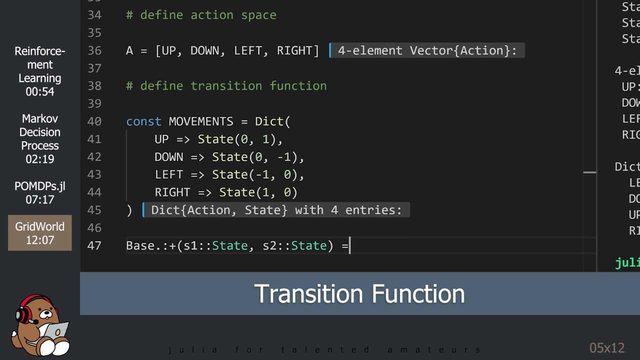 so brace yourself. We start by setting up a dictionary that maps each action to a new state, which defines movement. So that wasn't too bad. Now we need to add a new method to the plus operator so we can add a current state to. 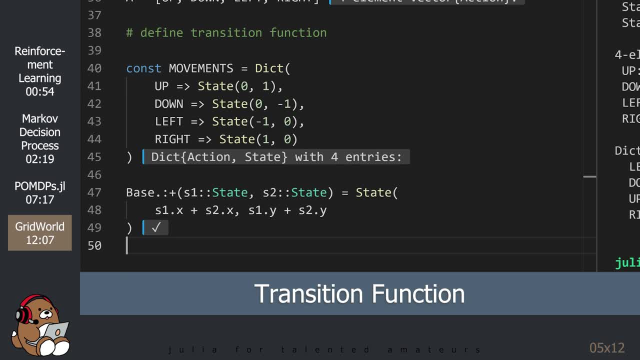 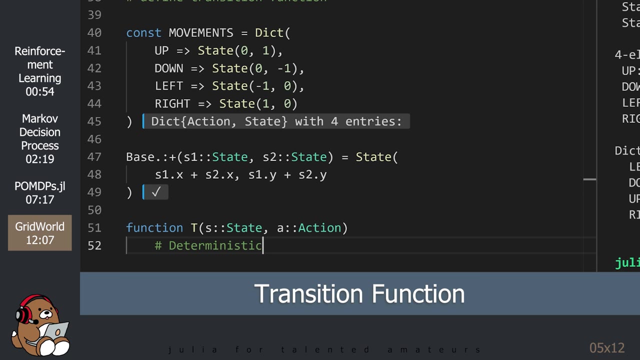 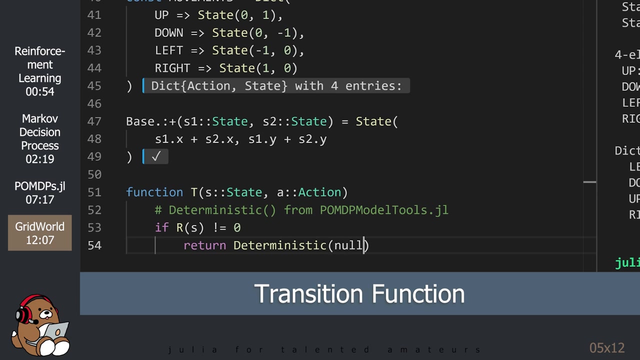 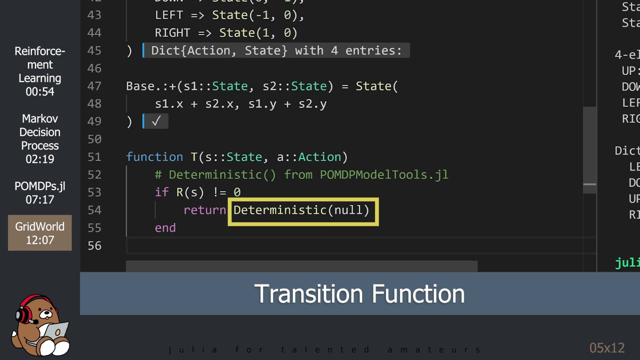 a movement in order to get a new state. So that wasn't too bad either. Now comes the tricky part. This is where we need to define a transition function, t, given a state s and an action a. The deterministic function is from the pomdp-model-toolsjl package and, according to their documentation, 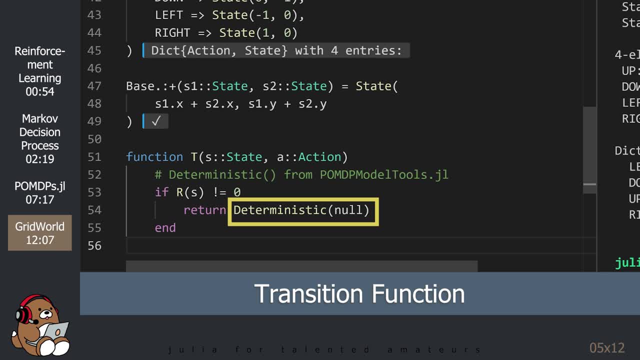 the deterministic function is intended to be used when a distribution is required, but the outcome is deterministic. So in this case, the variable null is state, which is used to end the game. This code will end the game when the agent lands on a tile with either a positive or 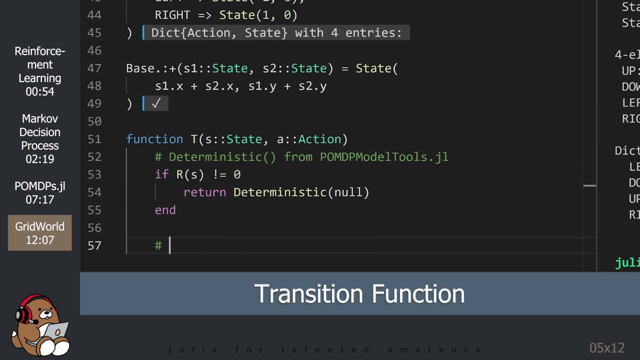 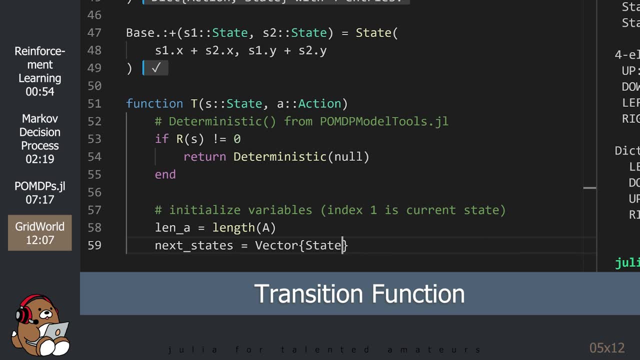 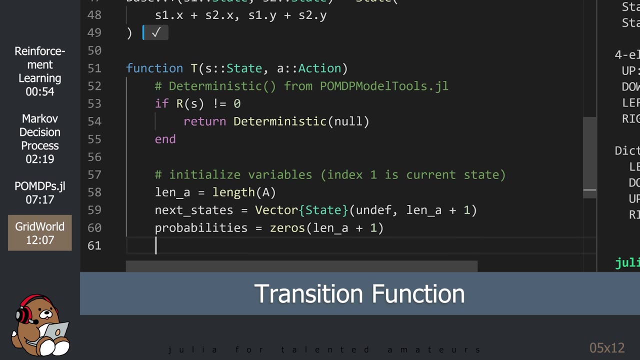 negative reward. Next, we need to initialize some variables. Next, underscore states is a 5-element vector initialized with undefined values. This vector will be used to contain the states needed for decision making. Element 1 is the current state and the other 4 elements are the 4 possible new states. 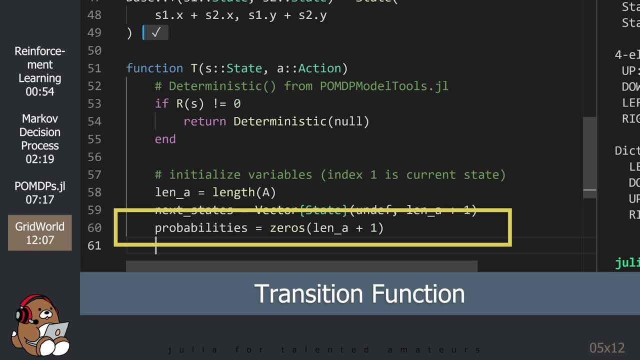 Probabilities is also a 5-element vector. Next underscore states is a 5-element vector initialized with undefined values. This is also a 5-element vector, but initialized with zeros. This vector will be used to contain the probability distribution of the agent moving in any given direction. 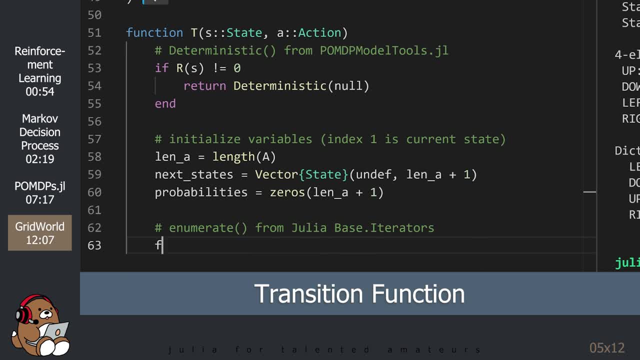 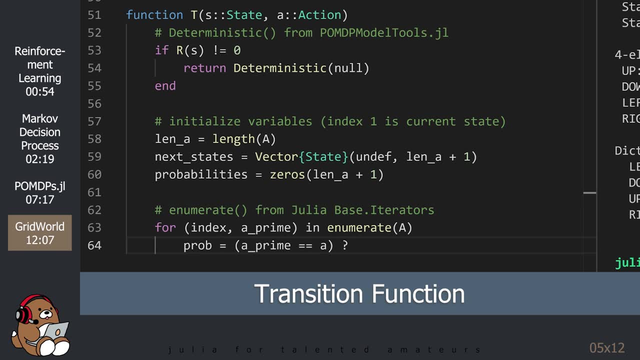 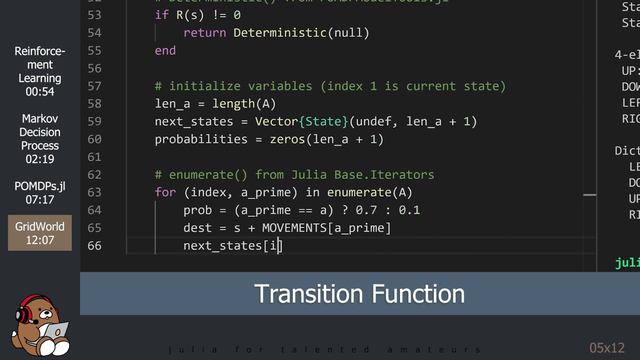 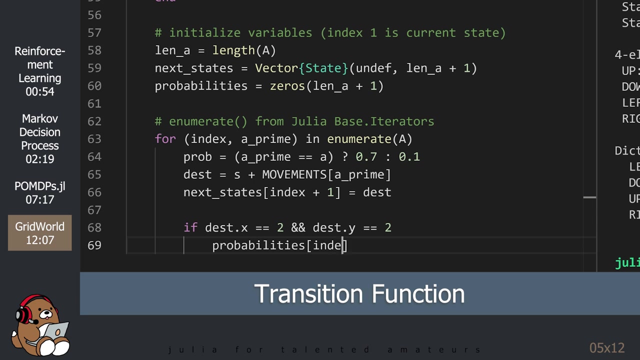 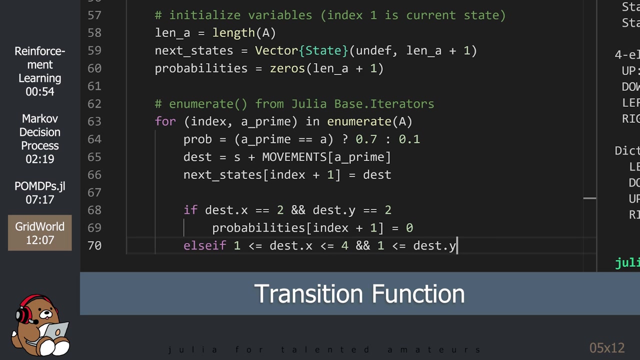 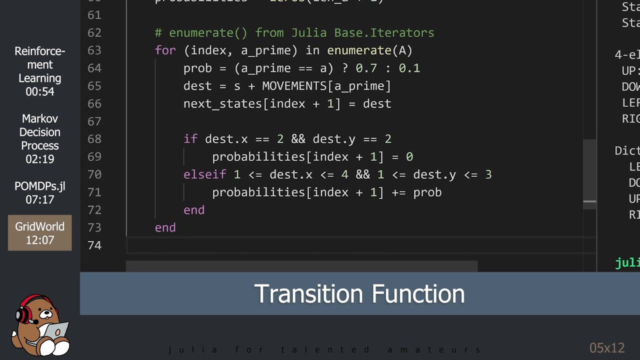 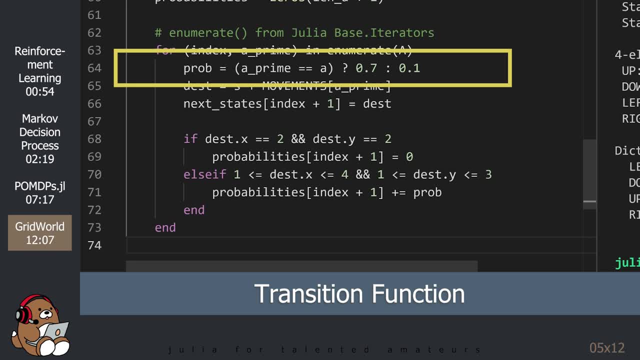 Using this code, we're saying there's a 70% chance that the Agent will move in the direction that it's supposed to move, but a 10% chance for each of the other directions. The if-else-if statement in the bottom half blocks the Agent from entering Tile. 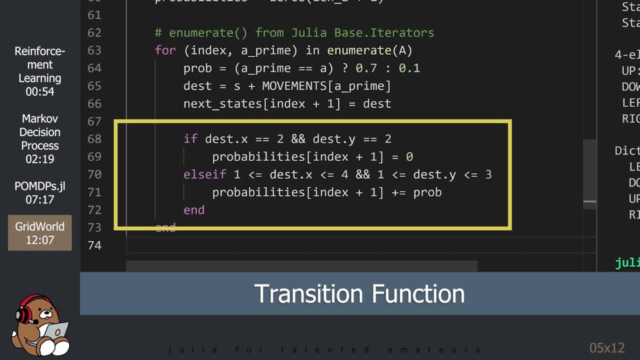 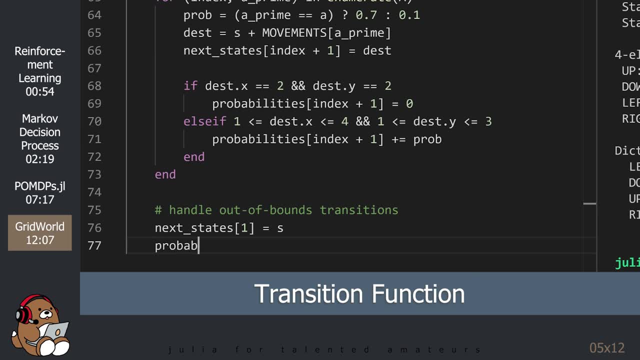 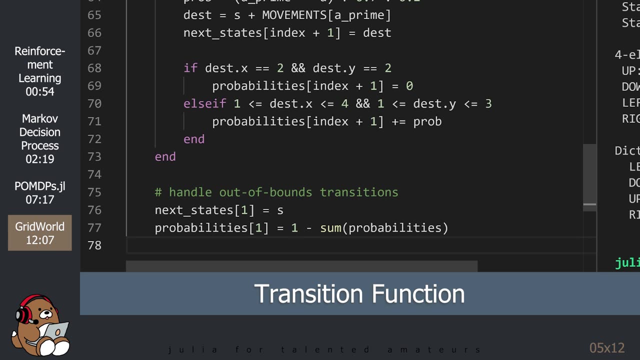 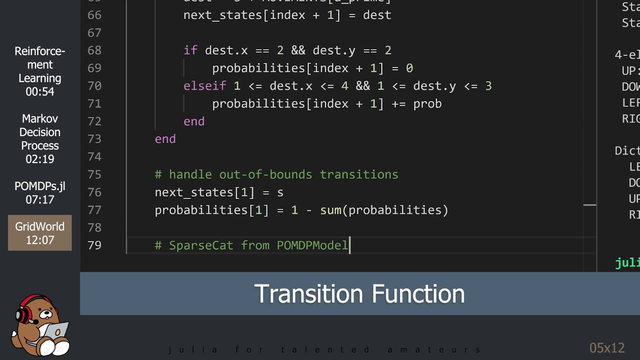 It also assigns probabilities for movements within the borders. This next section handles attempts by the Agent to move outside of the borders. This code makes the Agent bounce off the border and remain in its current state. This final section returns something called a Sparse Categorical Distribution, using the 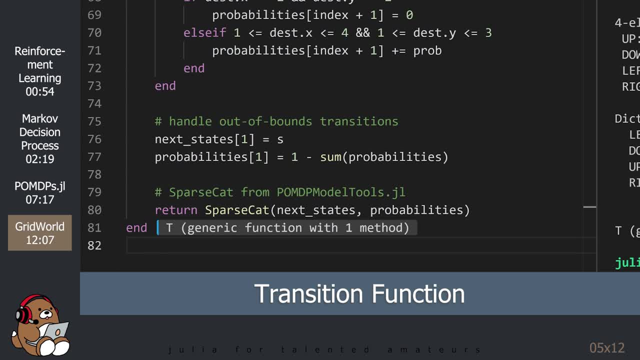 SparseCat. constructor from the pomdp-model-toolsjl package. SparseCat assigns the probabilities contained in the probabilities vector to the states in the nextStates vector. So that's a lot of code for just one function. If you're going to make a mistake anywhere in this tutorial, there's a good chance that. 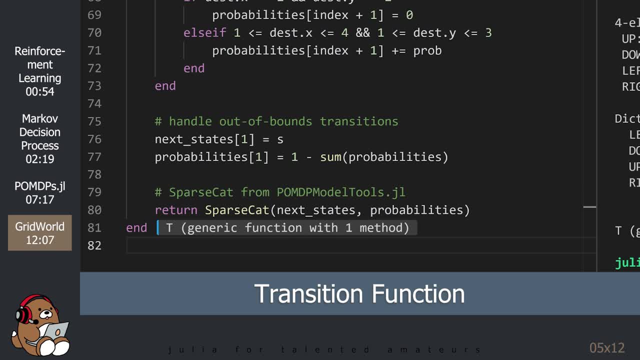 it will be here when creating the transition function, so be sure to double-check your code. You can find all of my code in my GitHub repository. There's a link to it in the description. The transition function is unique to the problem that you're trying to solve, so there's. 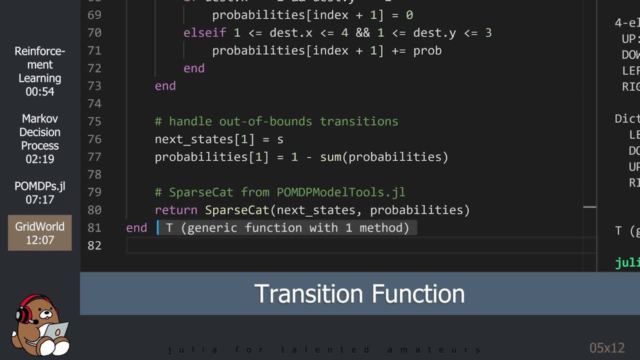 really no way to generalize it. Being able to write this code will test your general coding skills using Julia, So now you can see why I consider this an intermediate-to-advanced subject. The good news is that the rest of the code is not as tricky. 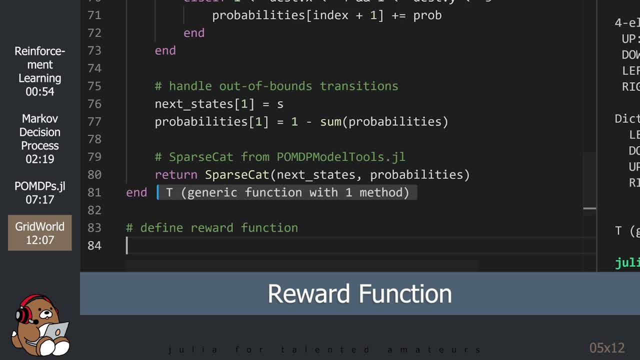 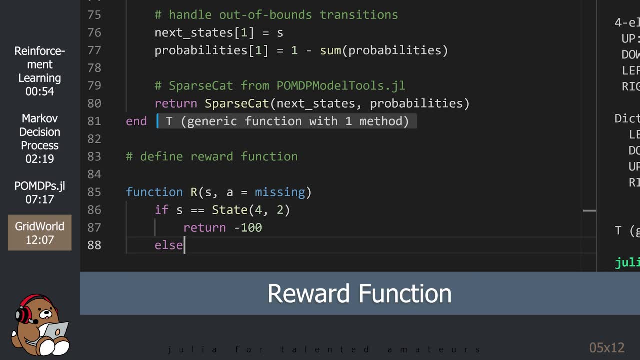 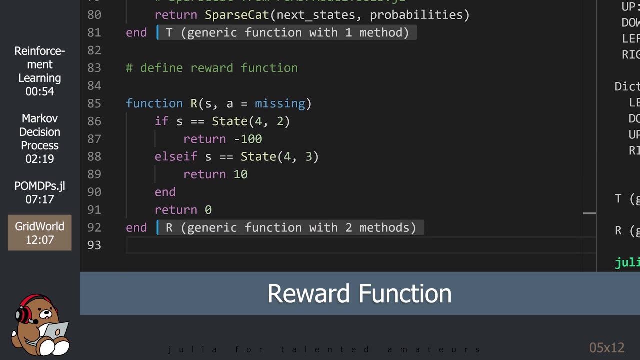 Next, let's define the code. Let's define the reward function. This code places a negative reward of negative 100 in tile for the LavaBits and places a positive reward of plus 10 in tile for the DoggoBiscuit. 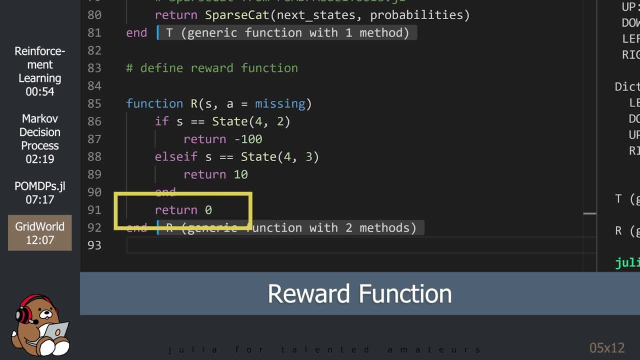 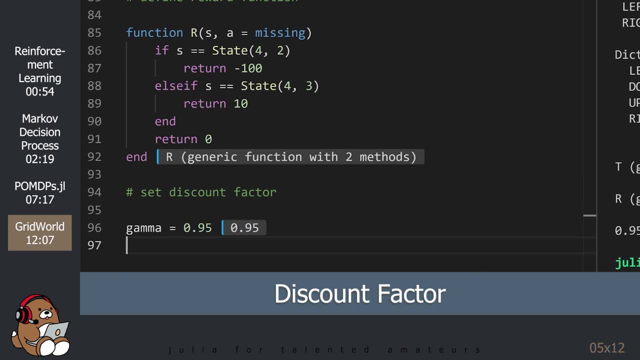 Otherwise, the reward in every other tile is zero. Next, we need to assign a value for the discount factor gamma. You may have heard the cliche that a dollar today is worth more than a dollar tomorrow. That's the idea behind the discount factor. 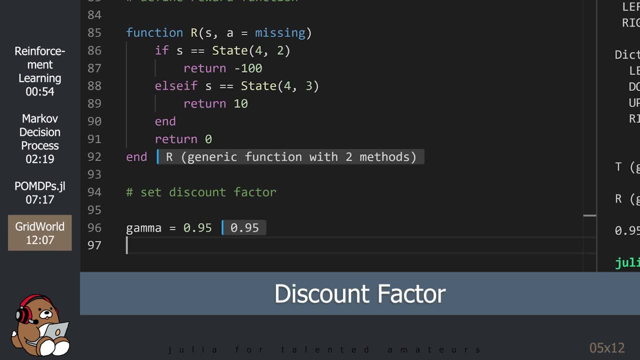 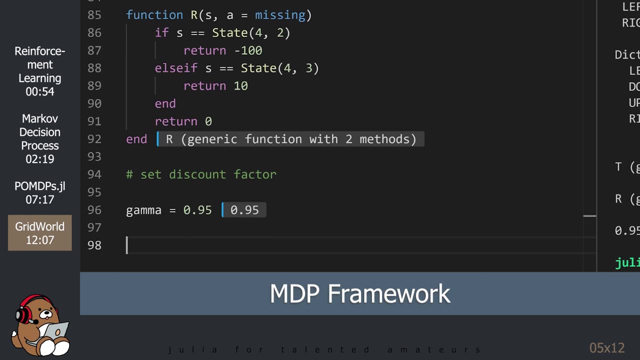 It places a higher value on near-term rewards and places a lower value on future rewards. I'm using a value of 95%, but you can use any value between 0 and 1.. Next, we need to define the MDP by using the QuickPOMDPs package. 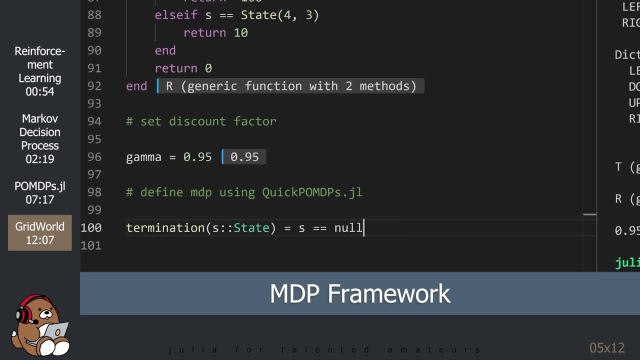 As part of the definition process, we need to define a function that returns a boolean for whether or not the state is the null state. We also need to define a function that returns a boolean for whether or not the state is the null state. We also need to define a custom data type for our environment, which we're calling. 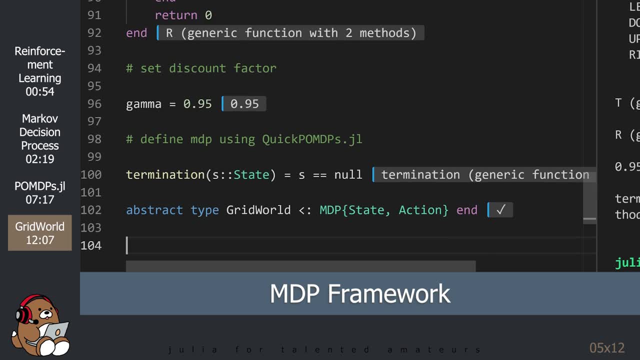 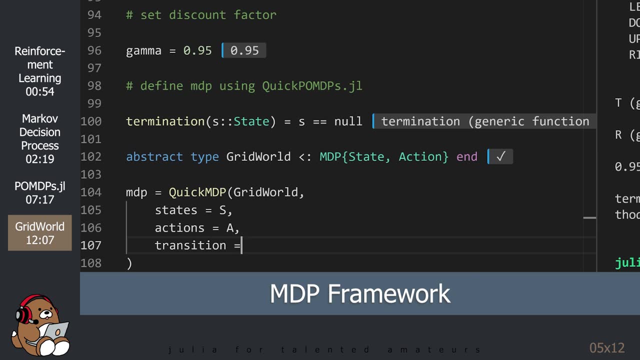 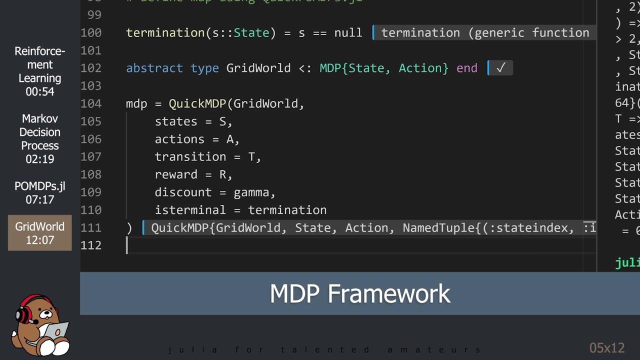 GridWorld. Finally, we use the QuickMDP constructor to create our MDP. You'll recognize most of the arguments from the mathematical definition of an MDP, which is a 5-element tuple consisting of S, A, T, R and Gamma. 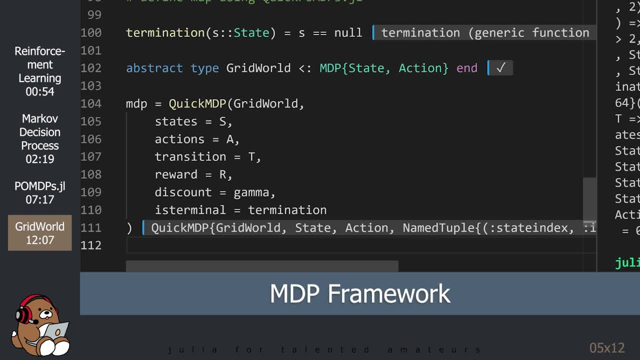 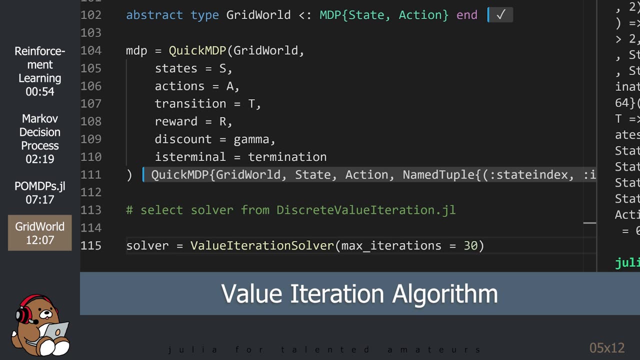 Using QuickMDP creates the mathematical framework that we can use to run through an algorithm. in order to quote-unquote- solve it. We're going to use a solver from the DiscreteValueIterationjl package, which is an implementation of the Value. 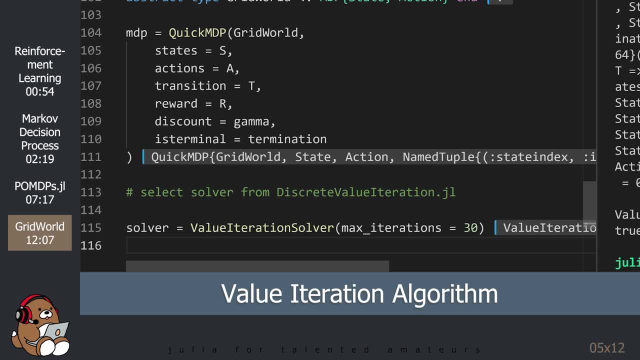 Iteration algorithm. You can play around with the maximum number of iterations, but 30 is fine for this example. As a reminder, the Value Iteration algorithm is based on the value iteration algorithm. You can play around with the maximum number of iterations, but 30 is fine for this example. 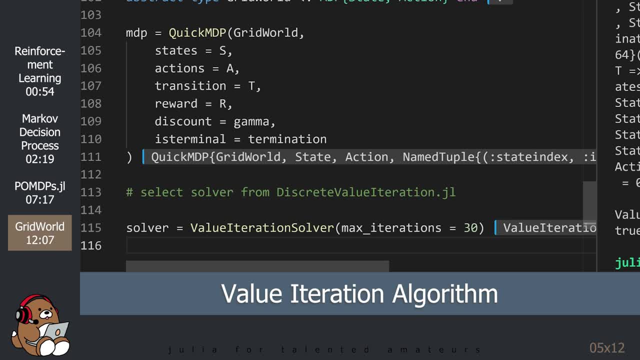 You can play around with the maximum number of iterations, but 30 is fine for this example. The Value Iteration algorithm uses an iterative process in order to calculate the value for each state, using something called the Bellman Equation. The Bellman Equation calculates the value of each state as the sum of an immediate reward. 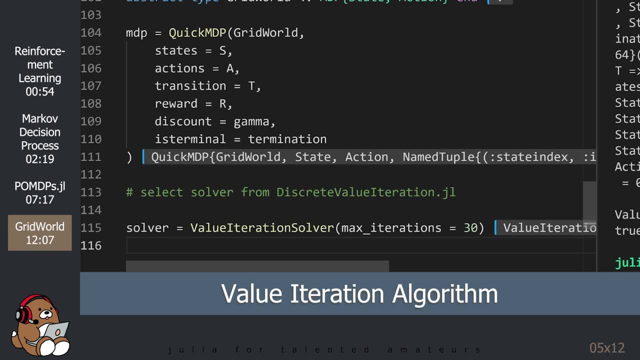 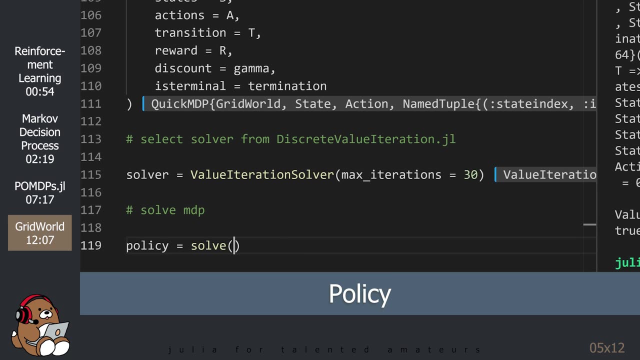 plus the discounted sum of all future rewards. By using this equation, the Value Iteration algorithm can figure out the optimal values for each state That maximizes the reward. Based on those values, the algorithm can then generate an optimal policy that maps each 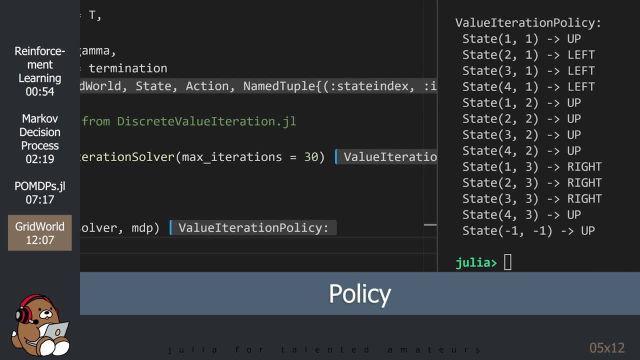 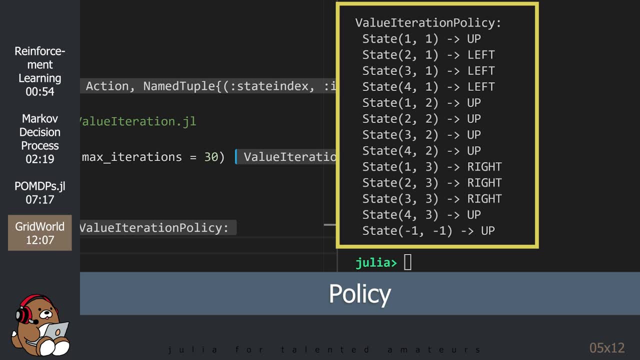 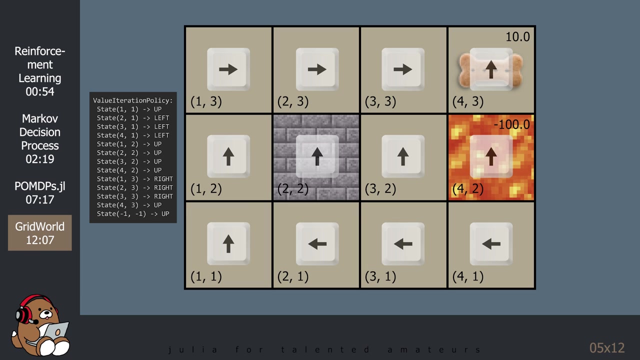 state to an action. If you look in the REPL, you'll see the actual policy. As you can see, each state is mapped to an action. Let's take a look at this policy applied to our diagram. So, according to this policy, if Agent Doggo starts in tile, then he should take. 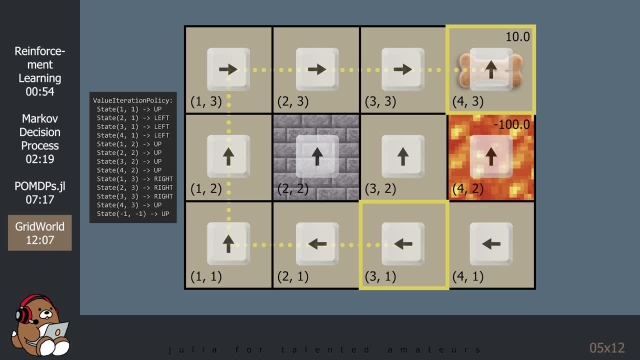 the long way around in order to avoid the lava pit By using this quote-unquote treasure map. no matter which tile our agent starts at, he will know the optimal path to take in order to get to the doggo biscuit. Pretty cool, right. 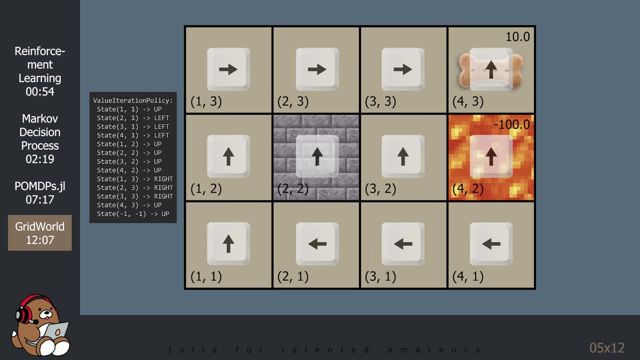 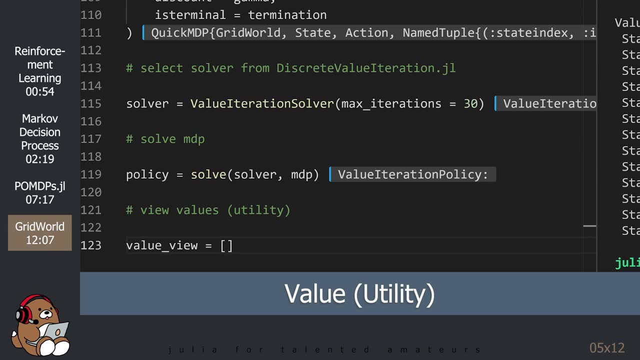 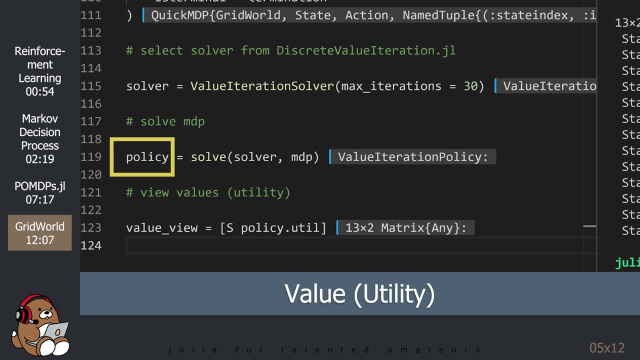 Now, how did the solver know? How did the solver know which actions to assign to each state? Let's go back to the editor and generate the values for each state. The variable Policy has several different fields, one of which is called U-T-I-L, which. 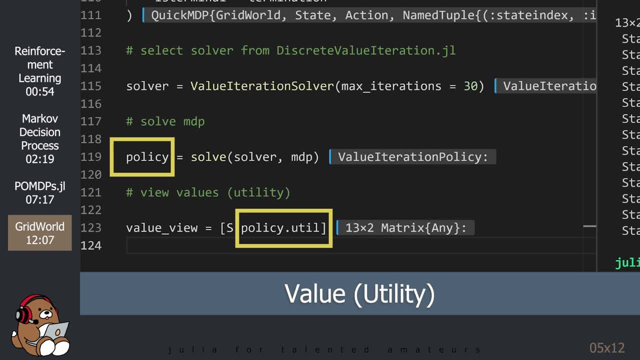 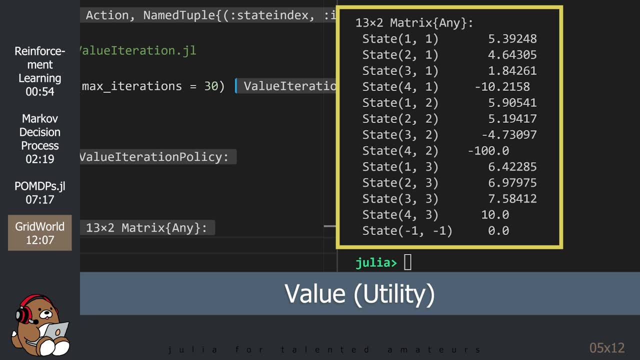 is short for Utility. Utility is another name for the values. If you look in the REPL, you'll see values of each state. By using these values, the solver can determine the actions to take in order to maximize the potential reward. Let's take a look at these values in our diagram. 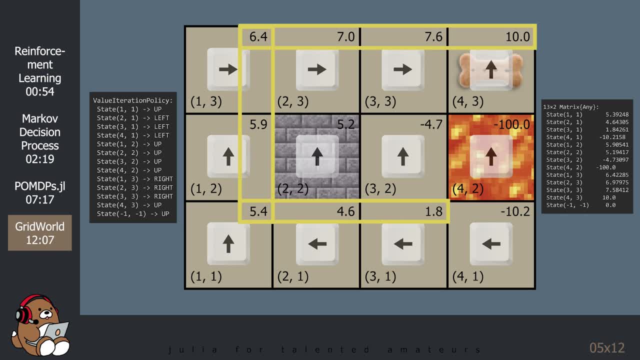 Now that we see the values, we can understand why it told the agent to go the long way around. State has a negative value, since there's a 10% chance of falling into the lava pit if the agent tries to move off that tile. 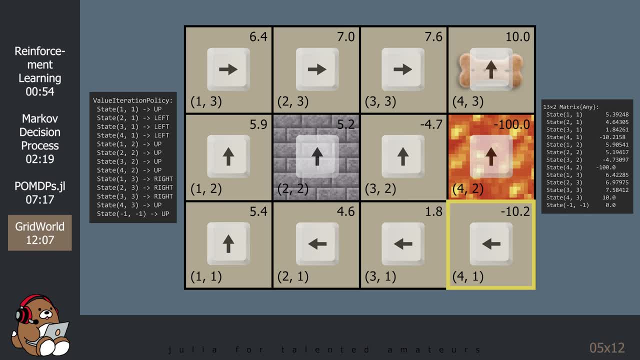 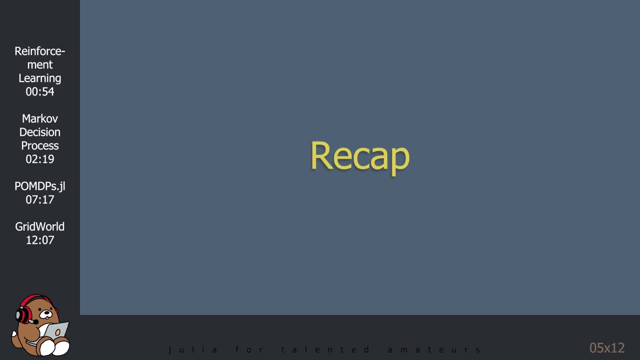 State also has a negative value for the same reason. Pretty amazing, right. We covered a lot of material in this tutorial, so let's break here and go through a recap of what we just saw. Today, we took our first step on our reinforcement learning journey. 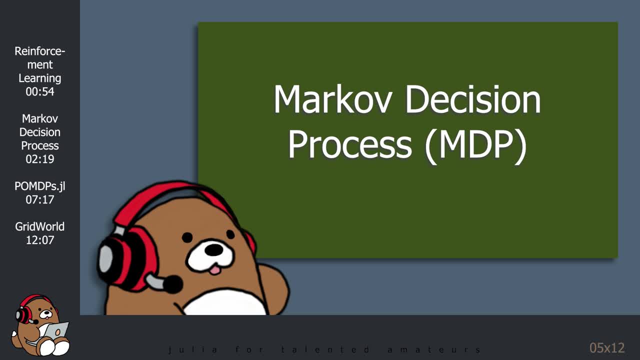 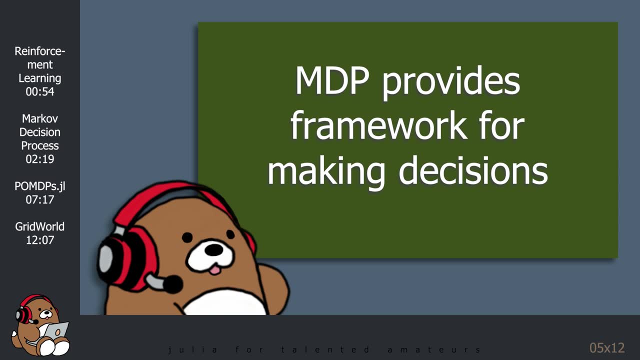 We've learned how to write our own reinforcement learning journey journey by learning about the Markov Decision Process, or MDP. An MDP is a mathematical framework for sequential decision-making under uncertainty. Mathematically, an MDP is a 5-element tuple containing S, A, T, R and Gamma, where S. 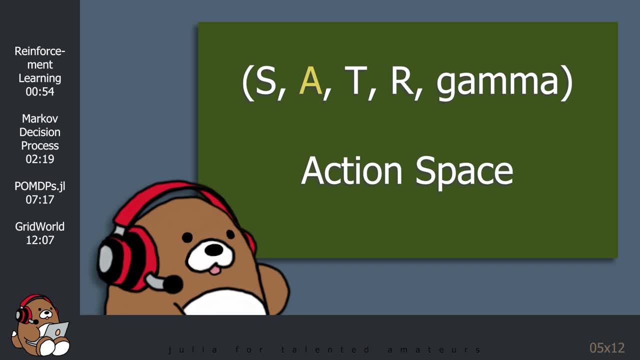 is the state, space A is the action, space T is the transition function, R is the reward function and Gamma is the discount factor. We solved our MDP using the Value Iteration Algorithm, which uses the Bellman Equation to figure out the optimal values for each state that maximizes the reward. 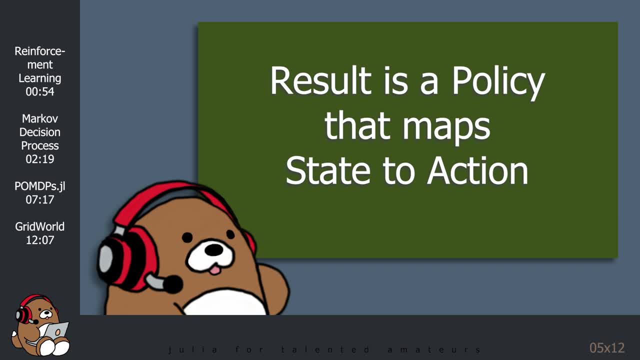 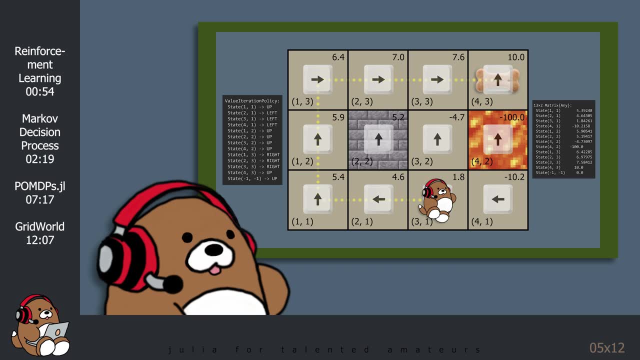 The result was a policy That mapped each state to an action. By using this policy, our Intelligent Agent was able to determine the optimal action to take given any state in order to obtain the maximum reward. That's a lot of concepts and code for one tutorial.